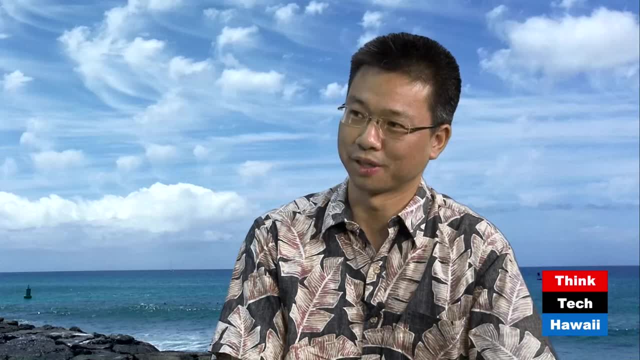 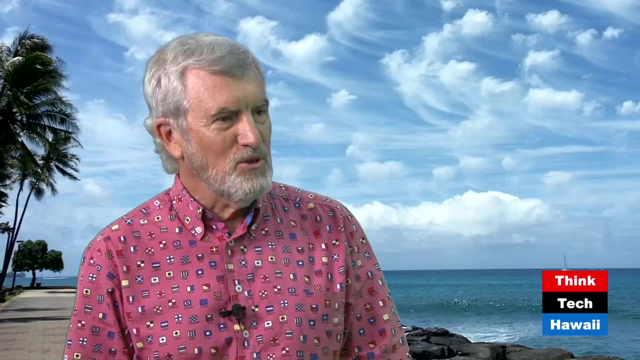 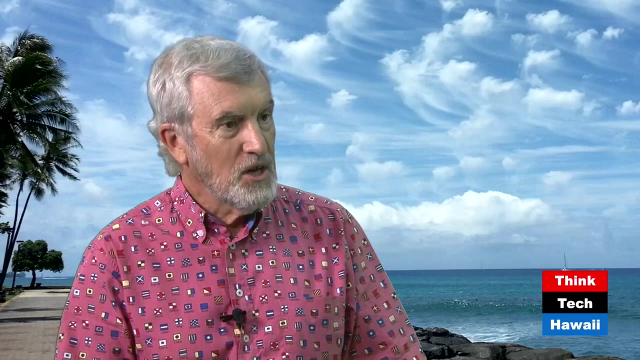 or the compositional makeup of the planetary interior. Okay, So this is really high pressures in comparison to what the general public would experience. It's not like just going down to the bottom of the ocean and the water pressure. This is really deep. This is hundreds of miles down beneath the Earth So we can actually 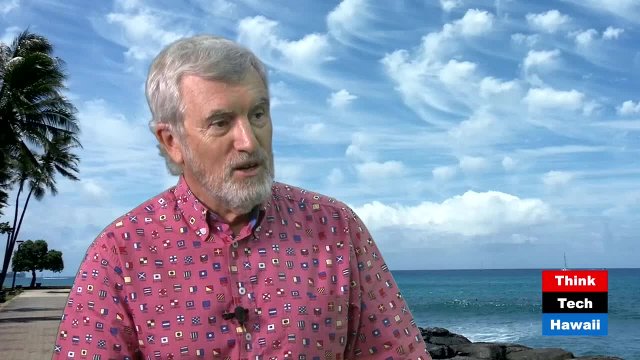 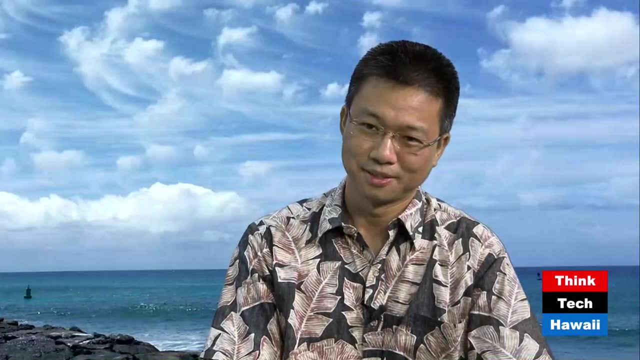 obtain the same kind of pressures and the same kind of temperatures, the same kind of temperatures that one would see inside the interior of the Earth. Is that correct? Yes, So using a device called a diamond anvil cell. so it's a pocket size, but we can squeeze. 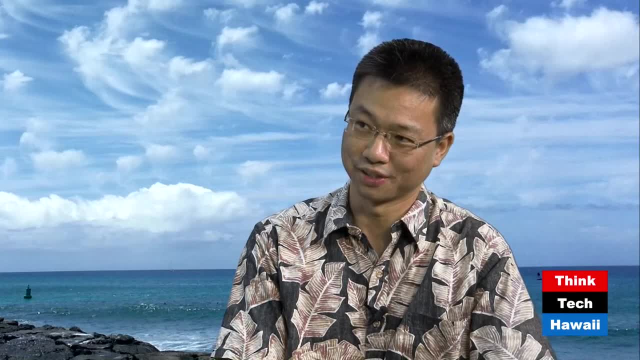 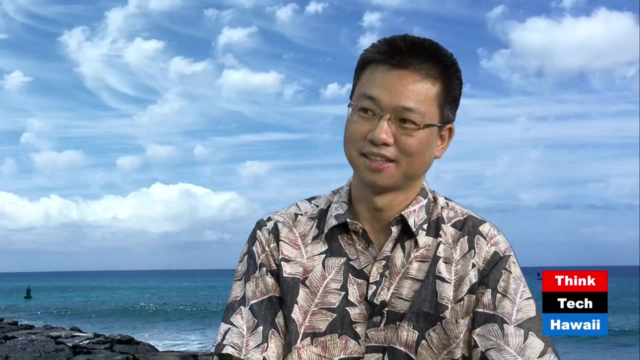 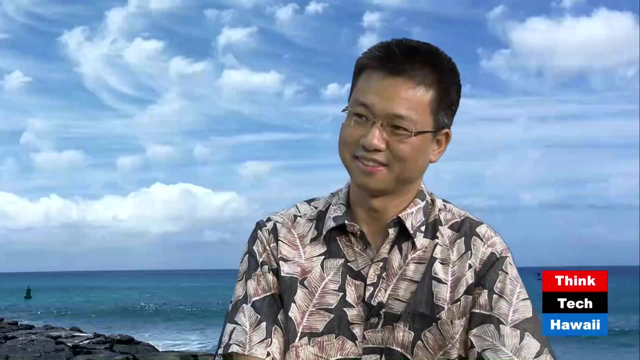 samples to the pressure temperature conditions found at the center of the Earth, so which is like more than 3 million atmosphere pressure, 3 million times the pressure that you and I are experiencing right now in the studio, for example. Yeah, exactly. And you mentioned samples. Are these big room-sized samples or are these little tiny things? It's very tiny sample because we know that the pressure is basically force over an area. So in order to reach higher pressure, we can either increase the force or we can decrease. 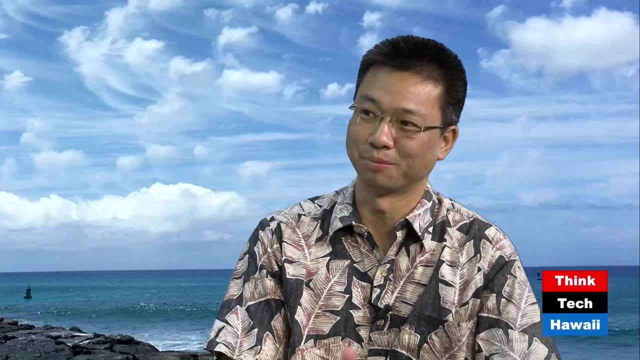 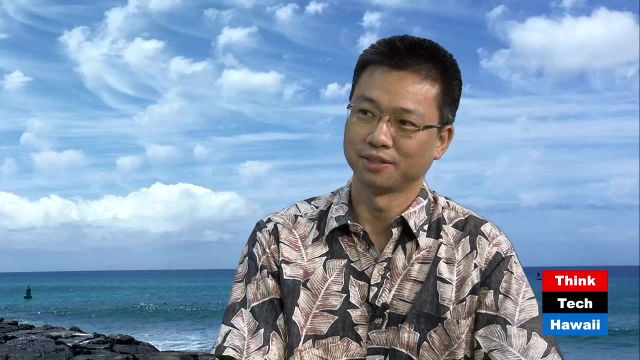 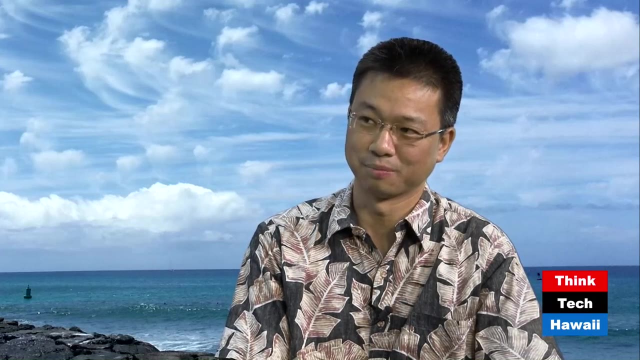 reduce the area that the background is in. So the samples are usually in order to reach the pressure of the center of the Earth. the sample volume is usually like tens of microns. Oh, very small. You can still see the sample, but only with a magnifying glass and that sort of thing. 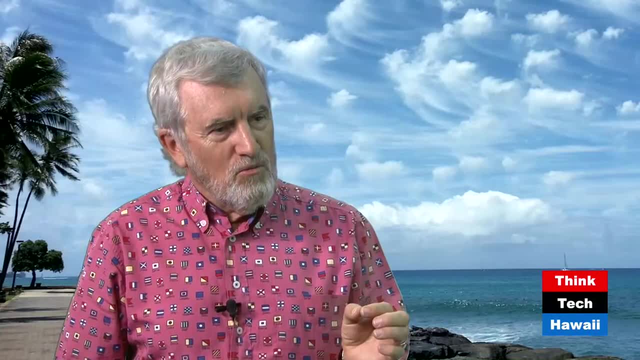 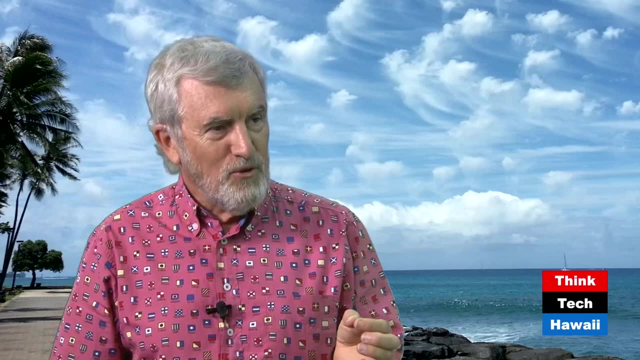 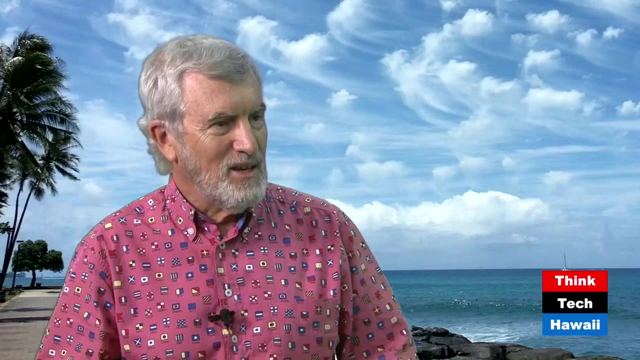 Yeah, Okay, and just to recap once more, we can do this to look at the minerals within the Earth, Mm-hmm. And along the first slide. if we can take a look at that, we can also apply this to the interior of any other planet. 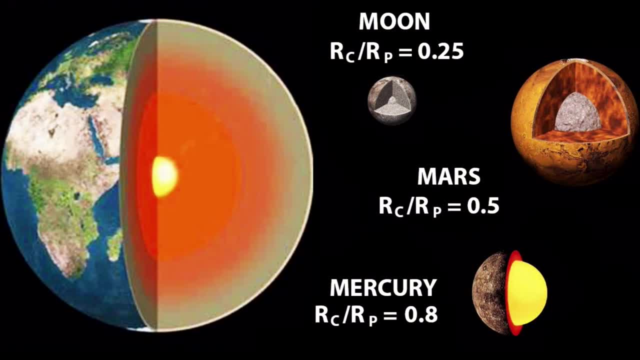 That's why you're in the Institute of Geophysics and Planetology: Yep, And here we're seeing the first slide with the Earth, and I guess these are all drawn to the same scale: Yep, Earth on the left-hand side, the Moon top center, Mars on the far right and the planet. 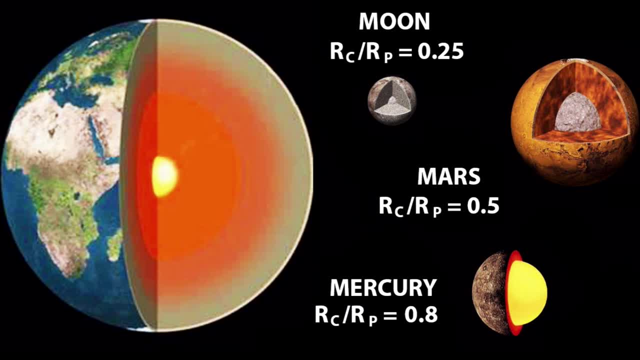 Mercury at the bottom, And we've got a ratio here: Rc over Rc, Rc over Rp is what? So it's the core radius versus the planetary radius, The radius of the core inside the planet. Yeah, over the radius of the planet. 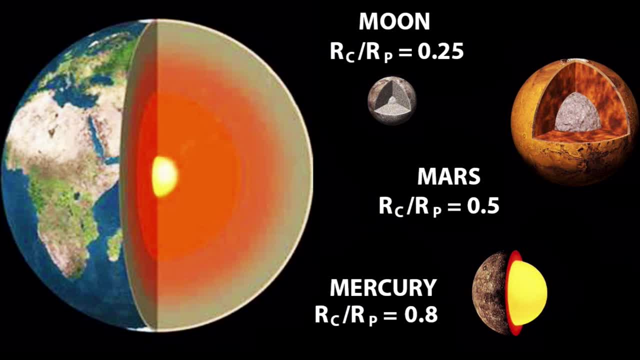 And what's interesting is that these numbers are different. right, Yeah, these are quite different. And then, so we know that the terrestrial-like planets, they all have a crust mantle and a core right, And then the Earth. 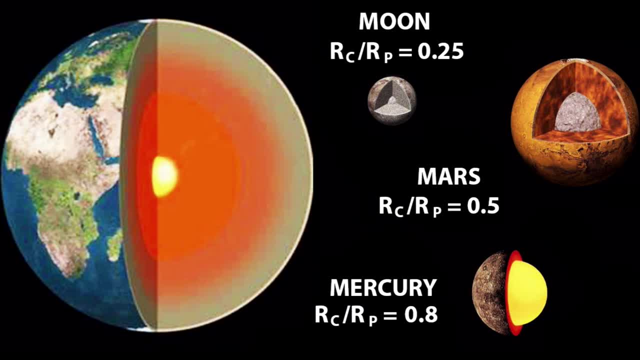 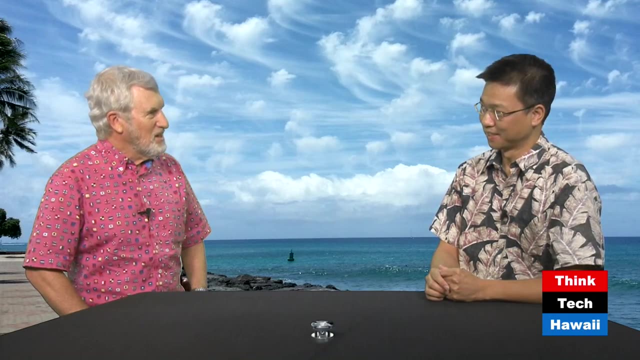 So the Earth has a core. So the Earth has a core. So the Earth's core is 2,900 kilometers in depth. So we can reach the top of the Earth's outer core if we do a hole 2,900 kilometers deep. 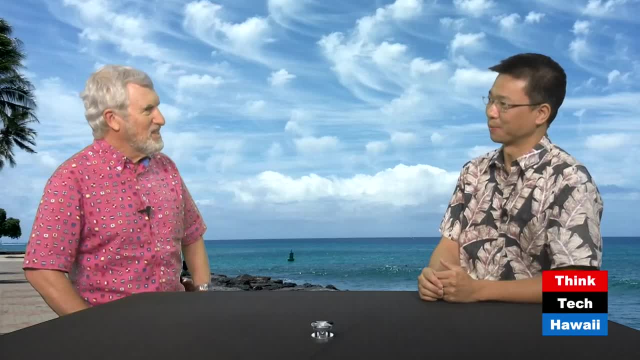 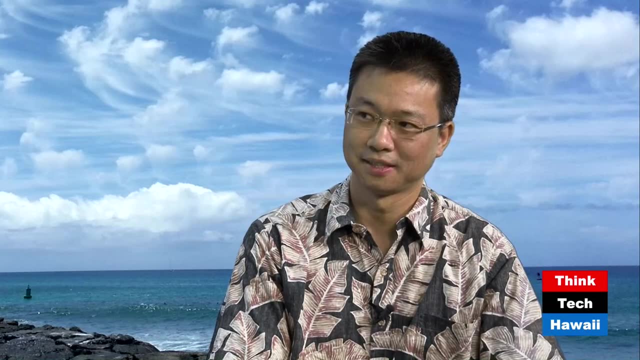 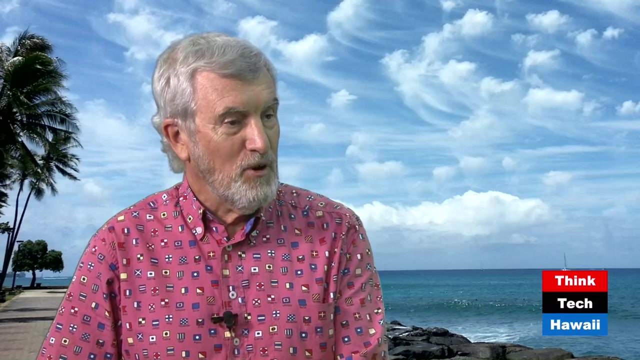 And then we can reach Impossible. but if we could, Yeah, that is of course impossible, But in our experiment we can really simulate the conditions at that depth. But the same experiments you're conducting, Yeah, You could also learn something about the interior of our Moon, or Mars, or Mercury, presumably. 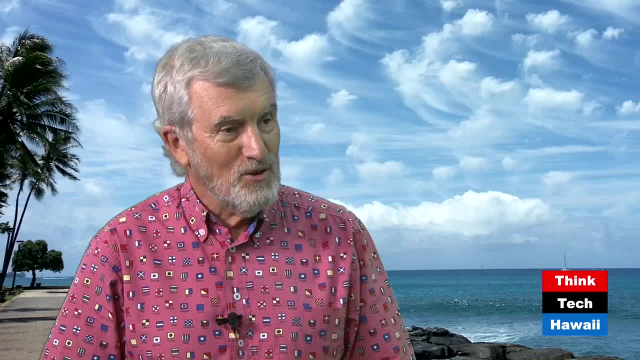 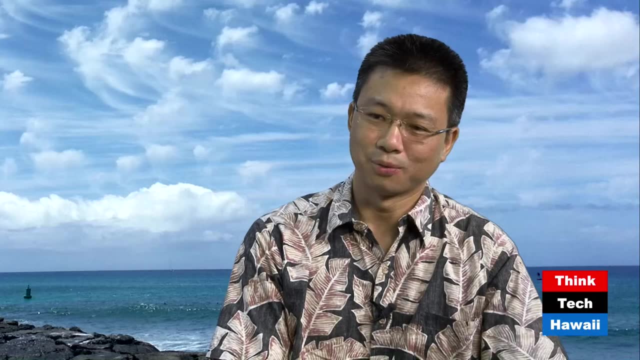 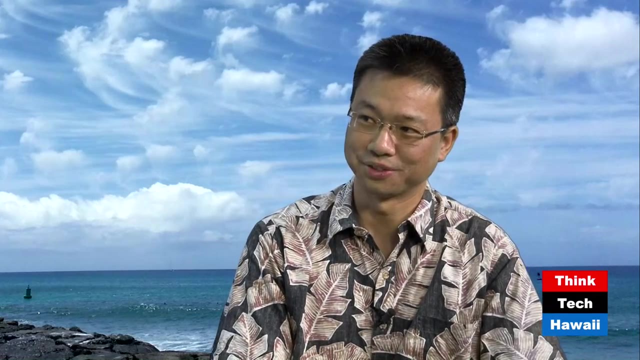 if you change the composition of the materials in your samples and that sort of thing. Yeah, We So currently So, yeah, so we are trying to understand. so what are the composition, makeup of this planet's cores? Right, So for the Earth core, there are many candidates, such as: 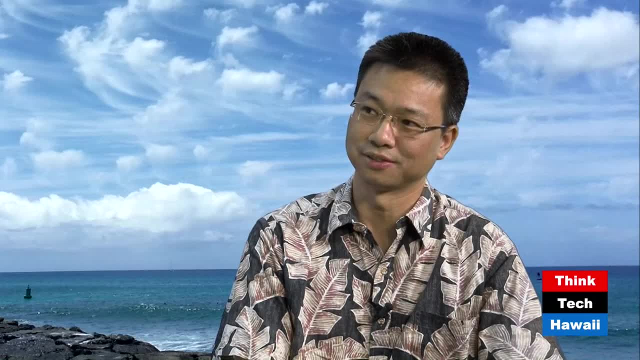 Yeah, Such as carbon oxygen like a. So the Earth core is mainly made of iron nickel. That's what we know, And for our dedicated viewers, of course, this is all background correct, Because Bin's been on the show at least a couple of times before. But you've just come back from Chicago where you've had like six weeks of experiments, So let's segue into what's new in your field, all right, So I think you went to the Argonne National Labs which we've got in the 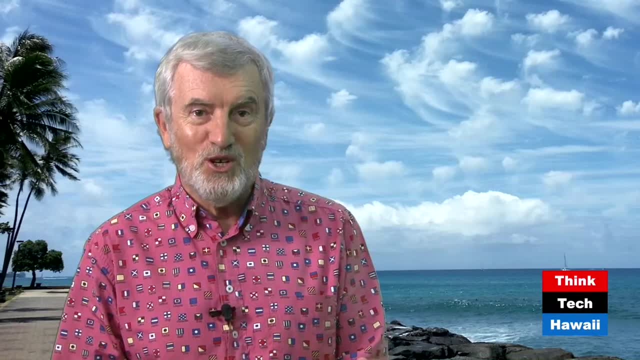 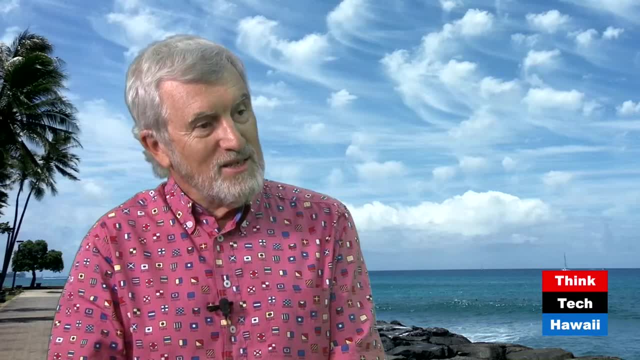 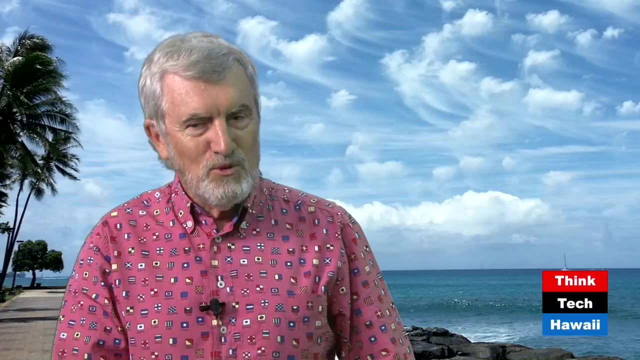 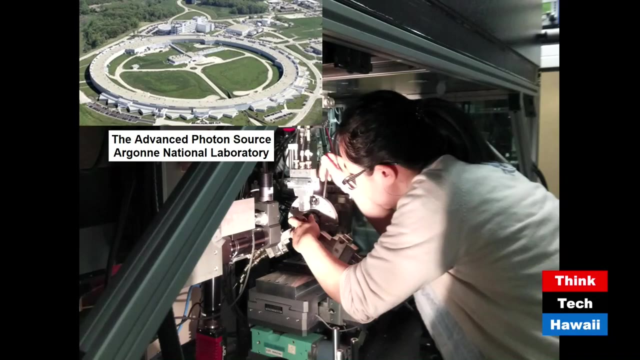 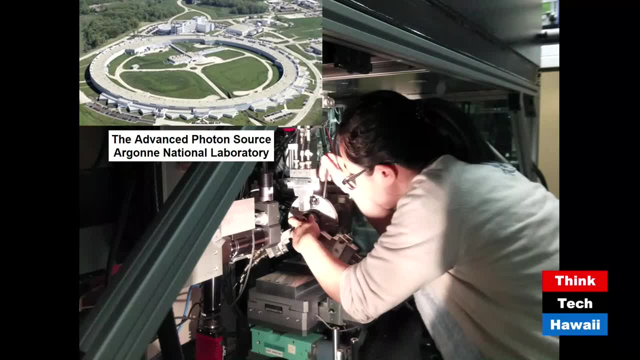 So in order to get the beam time in the advanced light source, we had to have our current bit apply in advance. we have to submit a proposal and then we can gather, sometimes like three days, sometimes six days in time. So I have six of them, like six of these proposals. 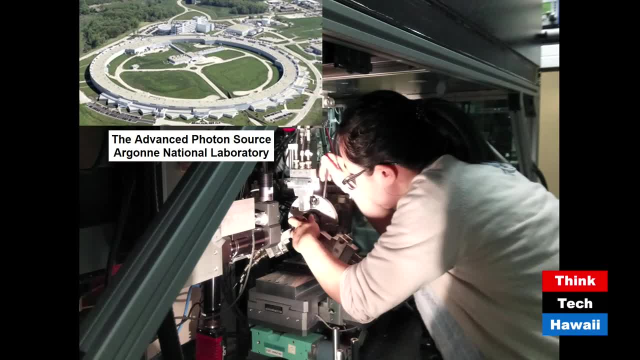 funded for the beam time And then? so what do we do? is that we are. we employ the high brilliance and high energy access source produced by this accelerator, And in the image you're using some jargon here. let's explain for our audience. 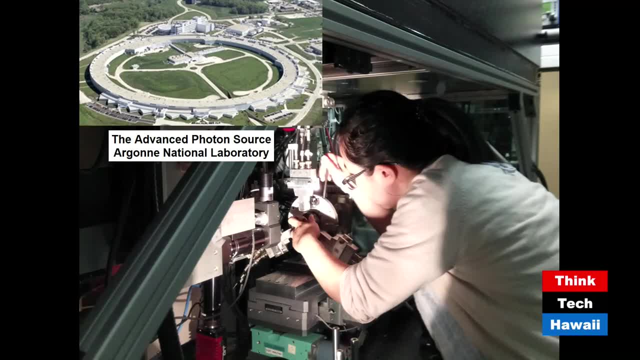 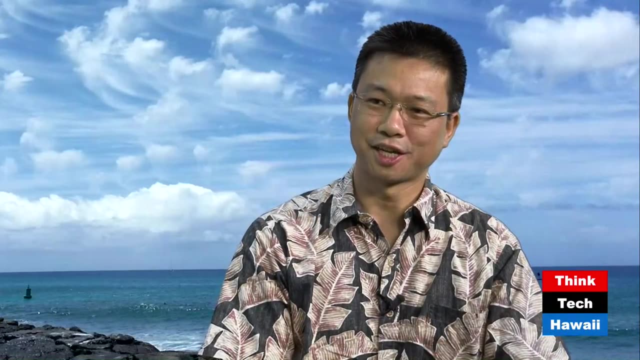 You mentioned beam time. Well, you went to this facility, which is outside Chicago, And the beam is that like a death ray from Star Trek, or what do you mean by beam time? Yeah, the beam time is basically the time that is awarded to a PI. 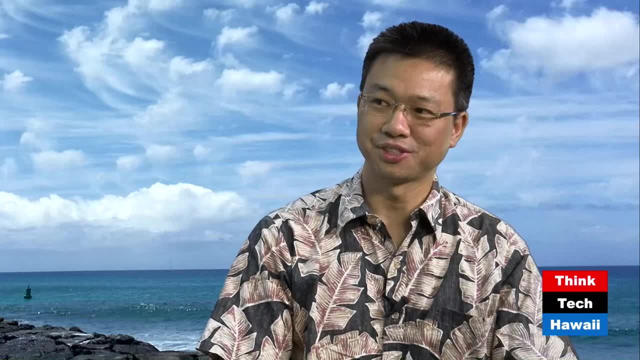 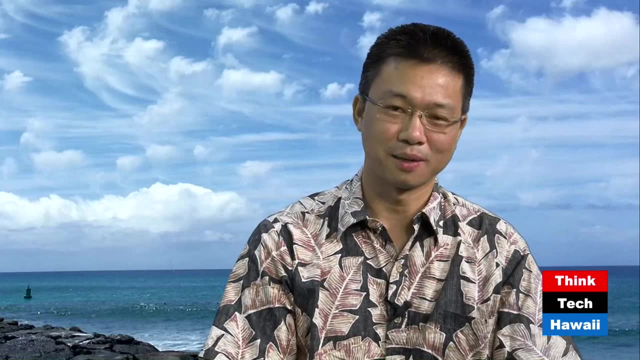 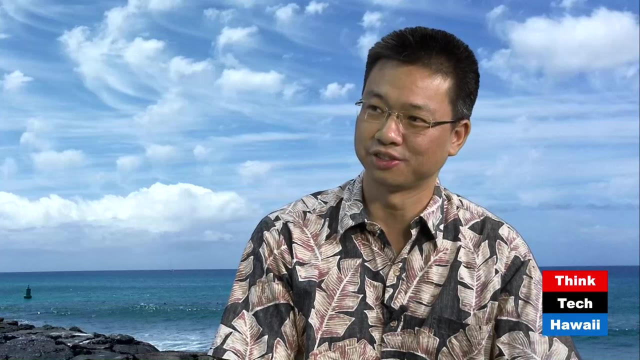 Principal investigator- Yeah, the principal investigator who can use the high brilliance X-ray? Okay, To probe your sample there. So there are many like beam lines. it's like a station, like more than 30 stations around the ring, So we only use a few of these stations. 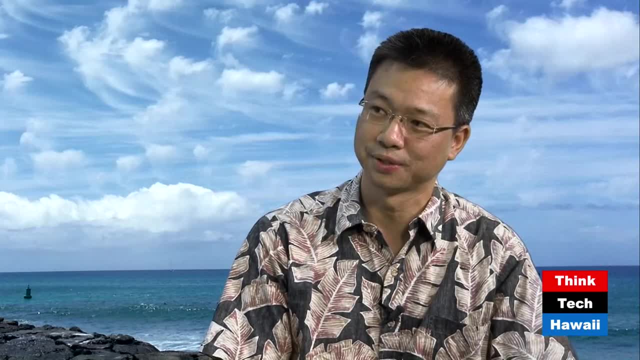 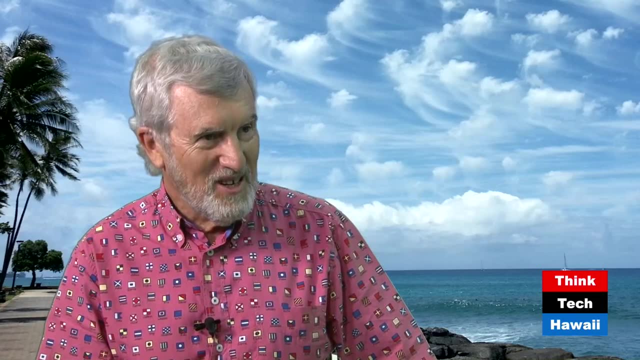 but there are some other stations that people use And you had to go to Chicago, presumably because those X-ray beams are not available here in Hawaii. No, it's not available here. It's not available here because it's highly energetic, right? 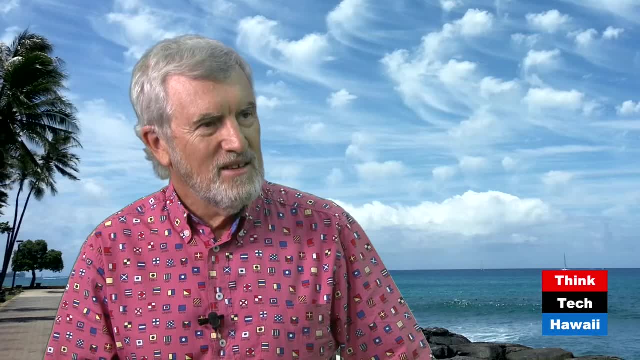 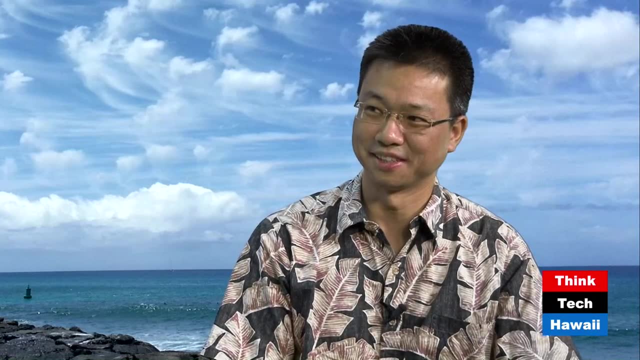 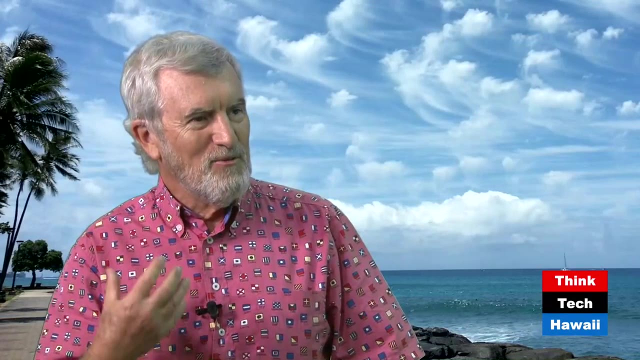 Yeah, because the brightness of the X-ray is close to the brightness of the surface of the sun, So that's really bright. And so when the audience hears you say you're using X-rays, this is not like the X-ray you would have when you go. 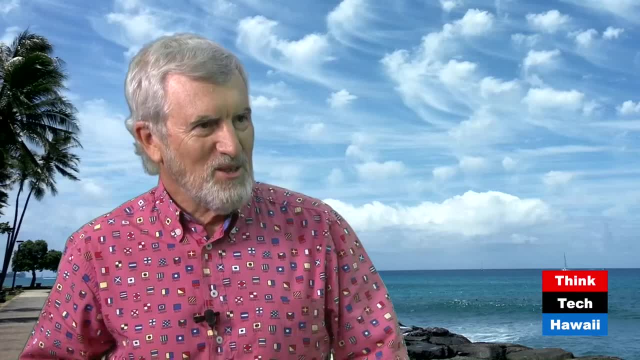 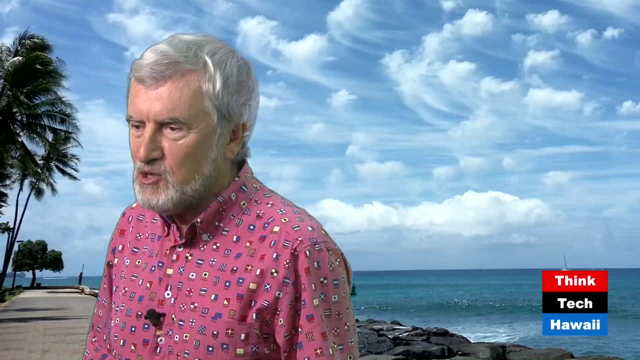 to the dentist to do your teeth. This is thousands, if not millions, of times more intense, correct? Yeah, it's much more intense. Nice, yeah, And let's take a look back at that The same image, because you're working on some equipment here, correct? 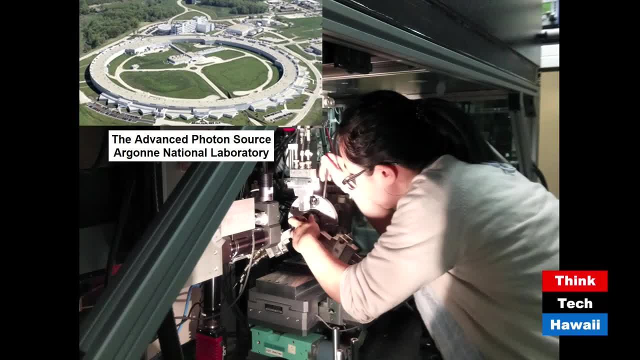 Yeah, So this is the experiment that we conducted employing the techniques available at one of the stations for the experimental touch at the Argonne National Lab. So this picture shows my student, Xiaojin Lai, working in this touch. She was trying to install a diamond anode cell at the stage. 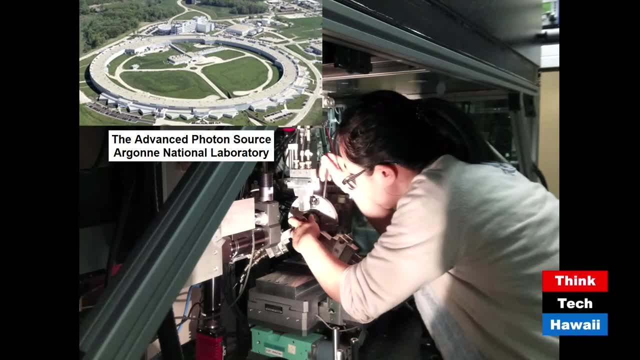 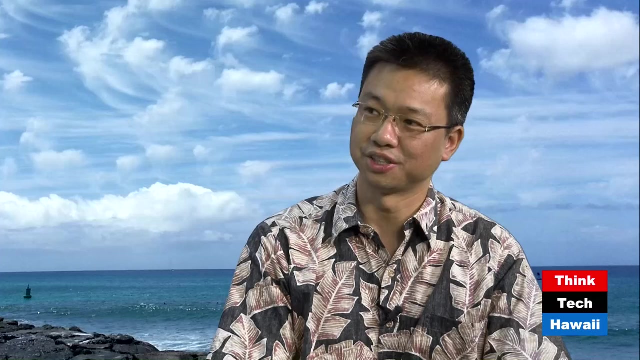 And then surrounding the diamond anode cell there are like three detectors that we used to probe the very weak signals from the sample. And then from the signals we can determine the vibrational and acoustic properties of the samples squeezed between two diamonds. Then we can determine the sound velocity. 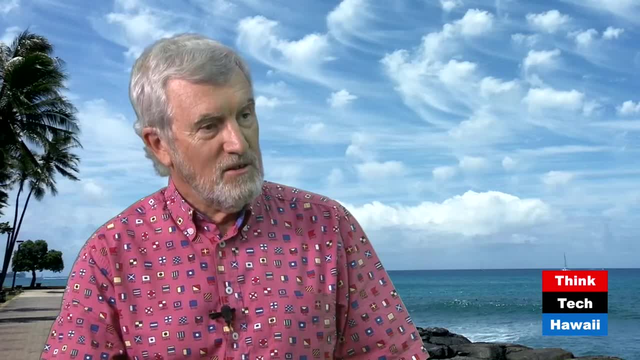 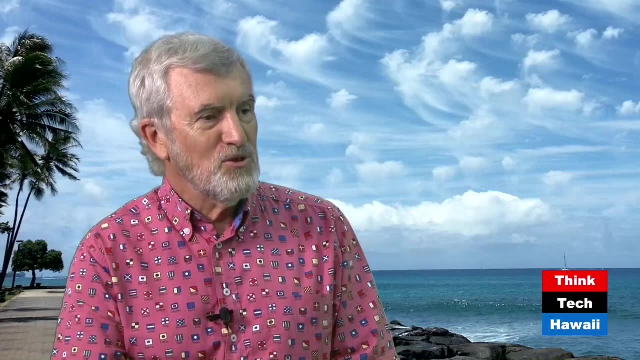 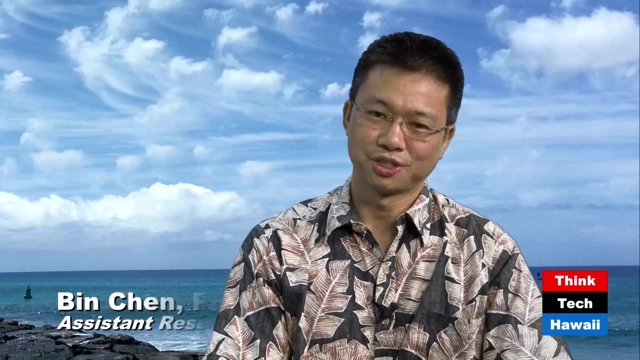 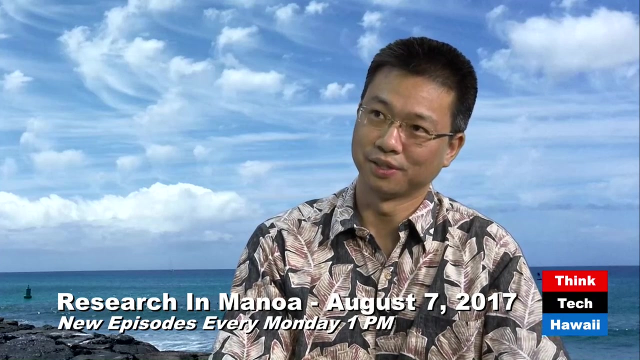 And this was a new project. You had to go there for six weeks, So can you tell us a bit about what was your objective to make this trip and to do this particular study? Yeah, this is a project funded by the National Science Foundation through the early career program. 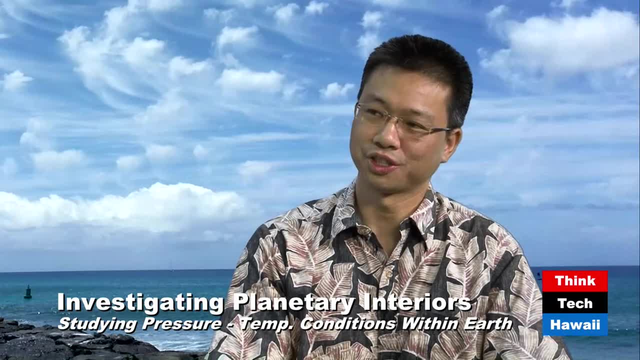 So it's a project. So it's a project funded by the National Science Foundation through the early career program. So it's a project funded by the National Science Foundation through the early career program. So the project is mainly about the sound and the lattice dynamics. 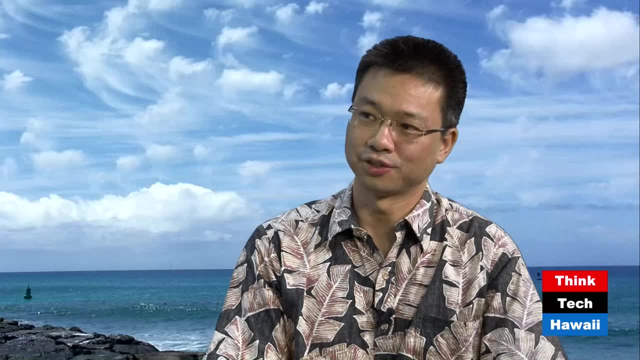 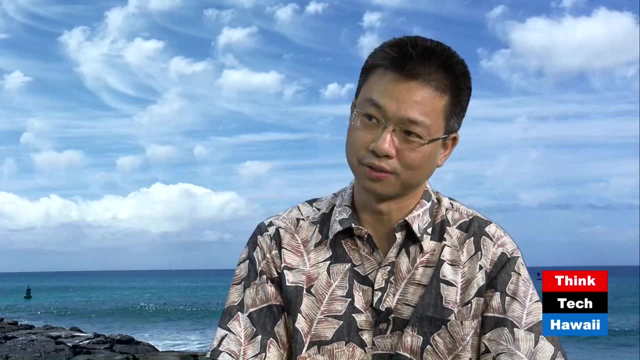 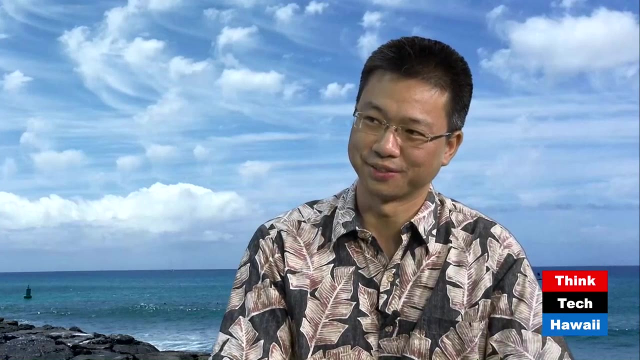 of iron alloys under high pressure in order to understand the composition and also the structure of the Earth's inns. So this is a five year project And then I have this funding. And you mentioned the National Science Foundation's early career award. And you mentioned the National Science Foundation's early career award. 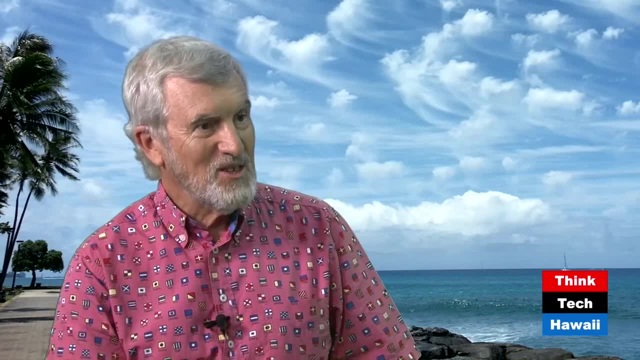 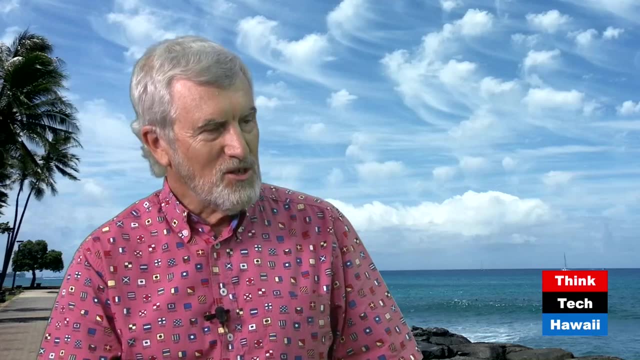 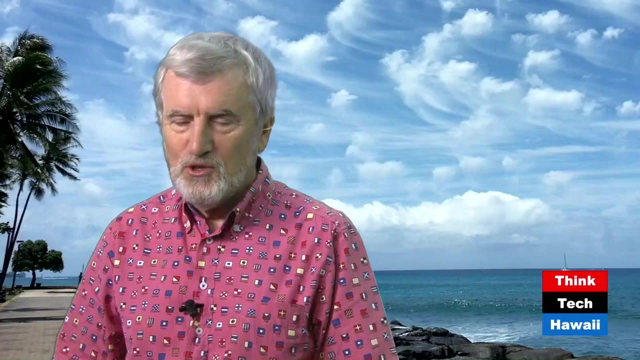 very difficult to obtain right and you managed to win such an award a year or so ago. my recollection so: congratulations on that year, and it's great to see that you've got students engaged already in training for next generation. let's look at the third slide, because that will show us a bit more of 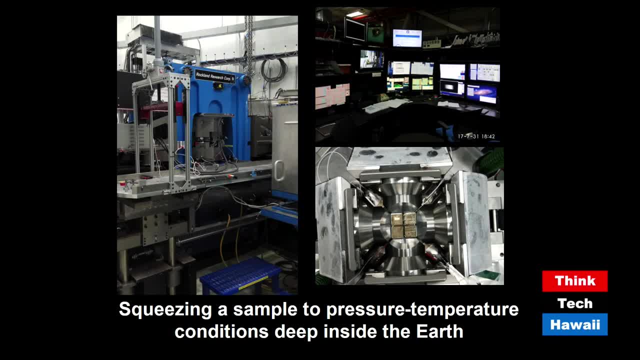 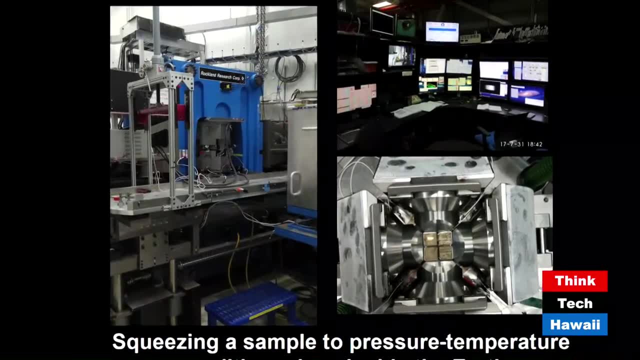 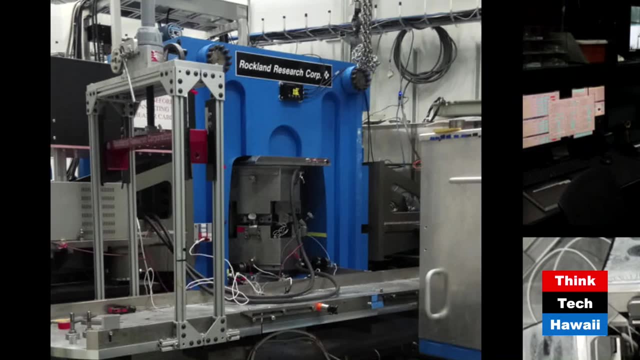 the, the equipment, I guess, that you're using. yeah, there's three images here. let's start with the blue thing at the left hand side. what is that? so this is a press that we use to squeeze large volume of samples under pressure, and we also heat it up. use this resistive heating method. so we have x-ray from the. 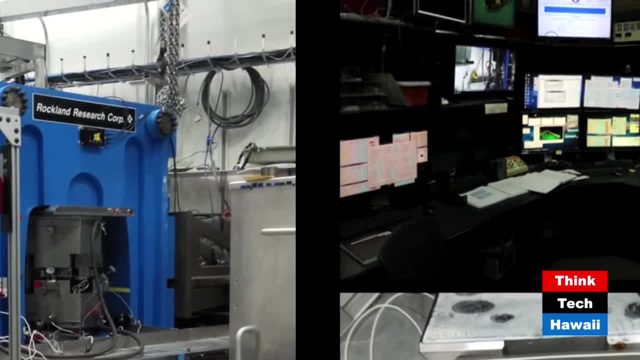 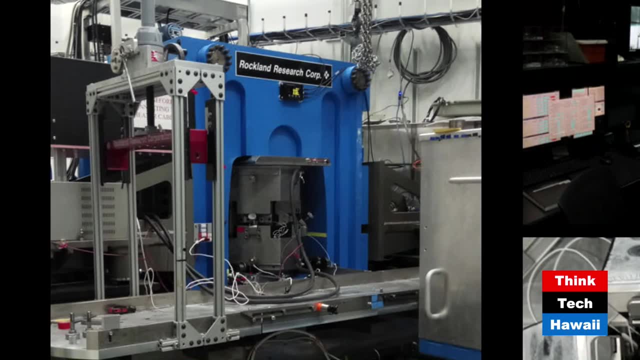 right side and then so the press is basically, because x-ray is stationary, we cannot move x-ray, we have to move this press. this press is uh, uh, it's a one thousand ton press. you can generally read the one thousand US ton. uh, that's one thousand tons, yeah. 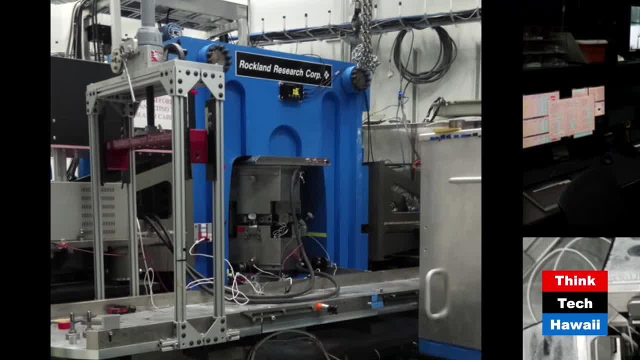 then we uh, so in the experimental hutch they can lift this full press off ground and move this press at the precision of micron millimeter level, like it's like a, yeah, micron level, okay, and uh the. the other image at the uh lower right of this slide, if we go right. 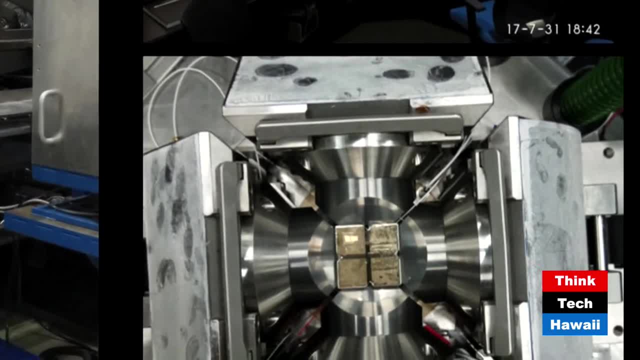 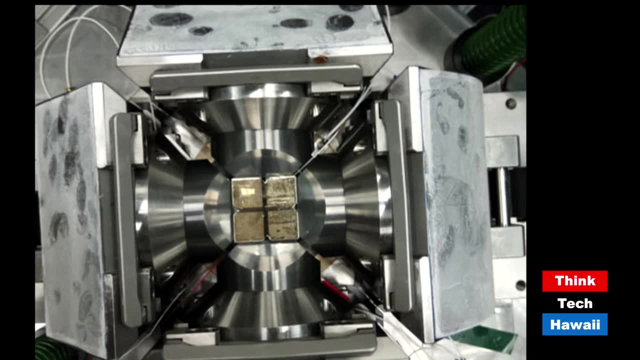 on this slide. this shows this is the uh, uh, the module we are using to compress our samples, so you can see that the uh, this, the center cube, is compressed from six directions. okay, and then four sides: top and bottom. yeah, both sides, and top and bottom, and then 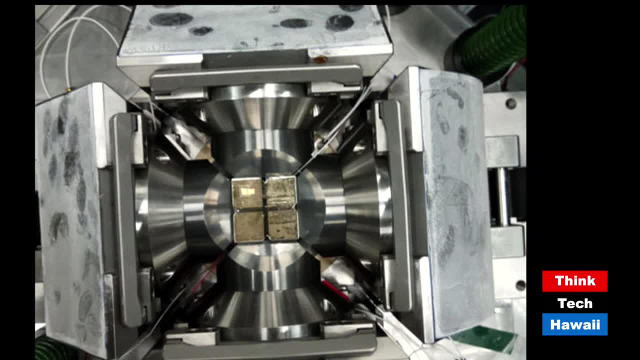 uh, our sample is located at the center of these eight cubes compressed by the form six directions. uh so, uh, in this experiment we actually acquired a new grade of constant carbide cubes. so we are trying to double the pressure capability of this large volume. press to like from 25 or 250 thousand. 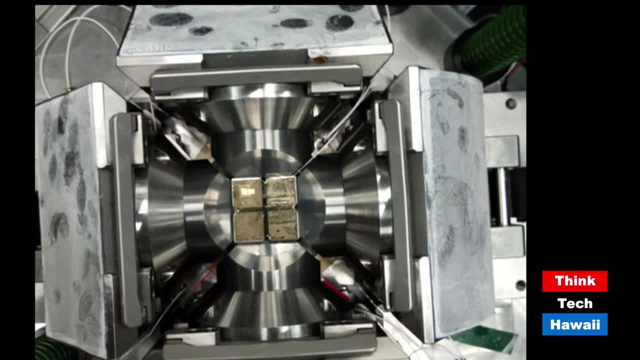 watts to 500 thousand and if you can increase the pressure then that's equivalent to going deeper into the earth. yeah, and you can do a lot of uh research using uh, this new grade of constant carbon, I see, and that new material is that developed in Hawaii or it's just a commercially? 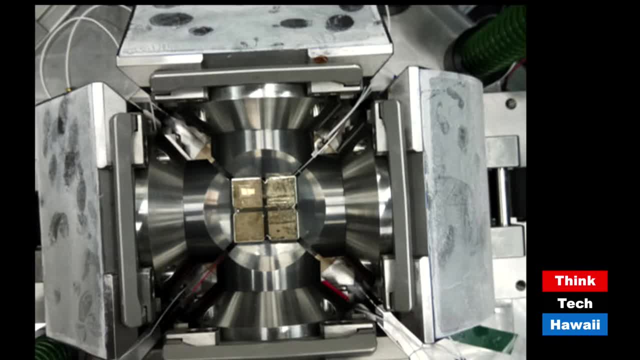 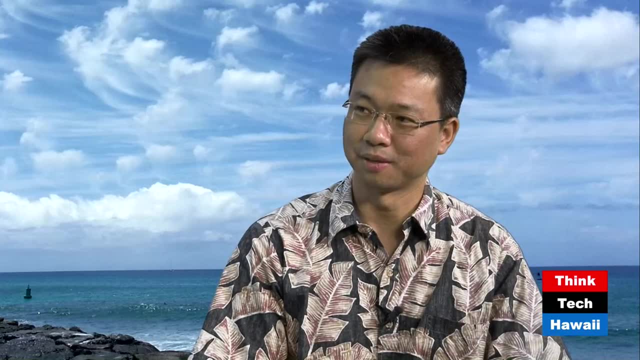 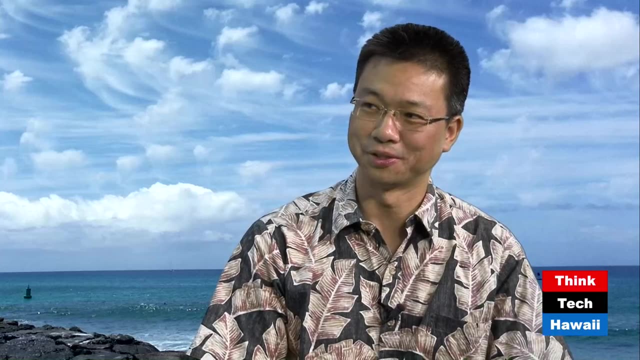 available. uh, it's developed in Japan. so Japan is quite advanced in the super hard material research. so they have this new grade of carbon. so we were quite lucky that we gathered these cubes and we want to double the pressure capability. that is can be achieved in- yeah, in the US, yeah, in the 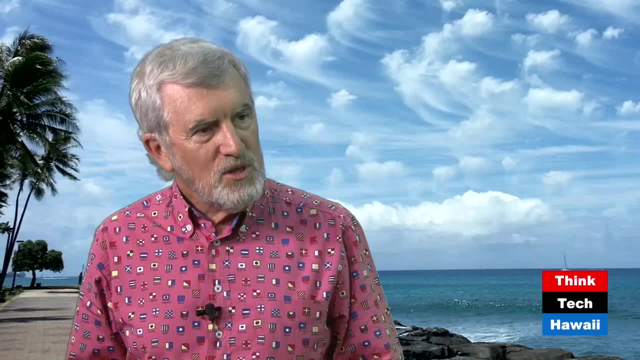 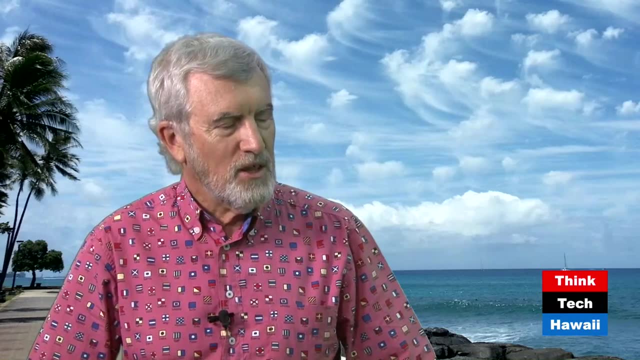 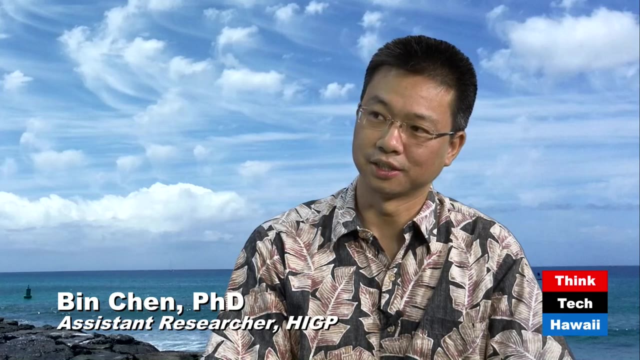 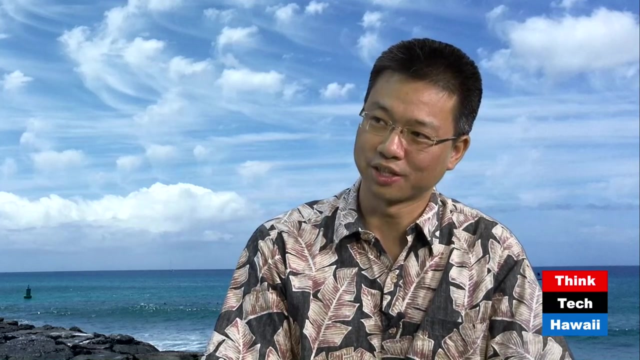 Japan. in Japan they have already done Argonne National Labs. is that the only facility in the United States, or are there others? or are there facilities like that in Japan or elsewhere? yeah, uh, in the, not a lot of them, like a number of them, like in the US in the West, uh, in the West Coast, as 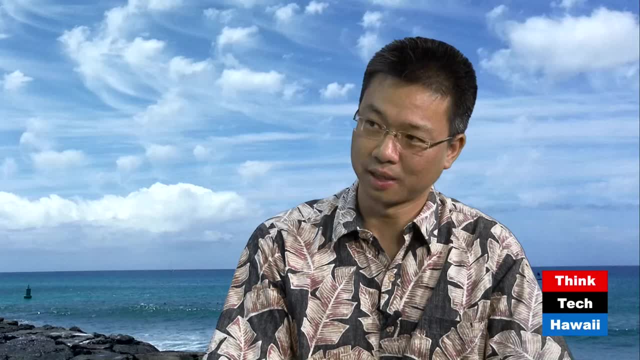 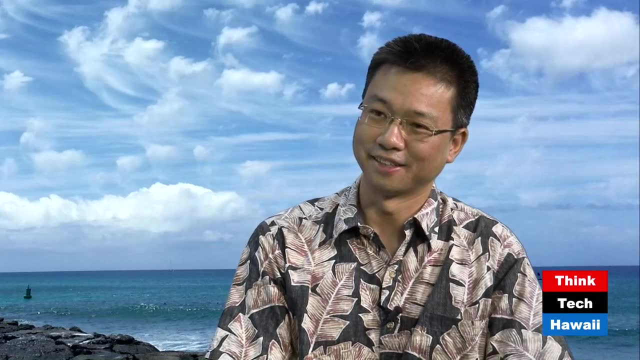 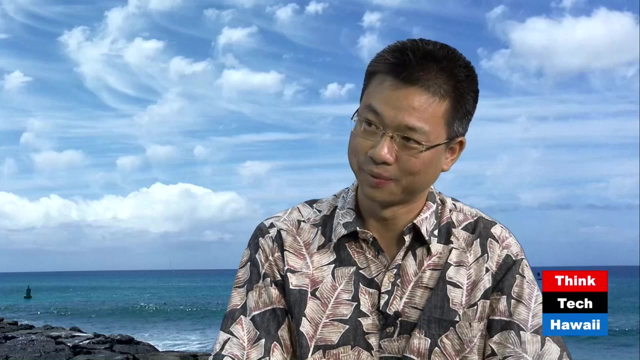 the other ones, the light source, the Lawrence Livermore National Lab, and then, uh, in the Midwest we have the Argonne National Lab, uh, and then in the on the East Coast we have is NSLS Brookhaven, and then in the West Coast we have the Argonne National Lab, and then in the West Coast we have 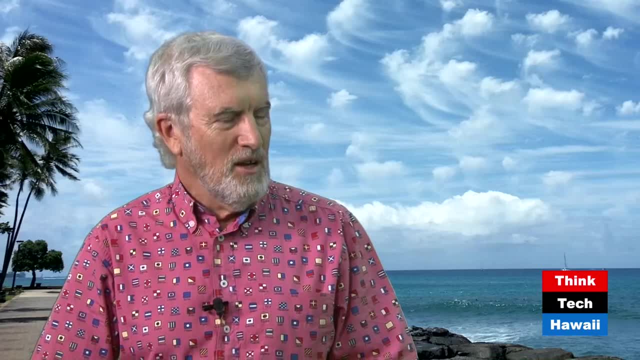 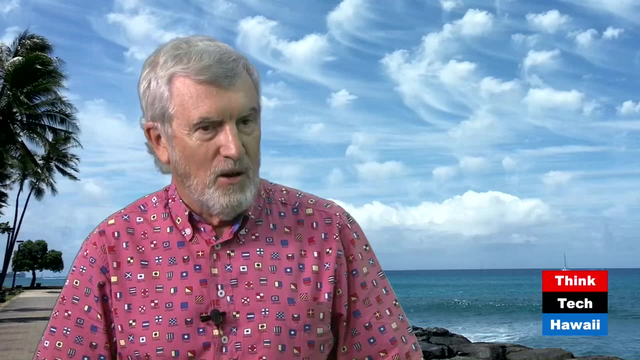 the Argonne National Lab and then in the West Coast we have the University of California. so we have two or three or four. and you said synchrotron. this is a facility that provides these high energy x-ray particles that investigators like yourself and our colleagues at the University 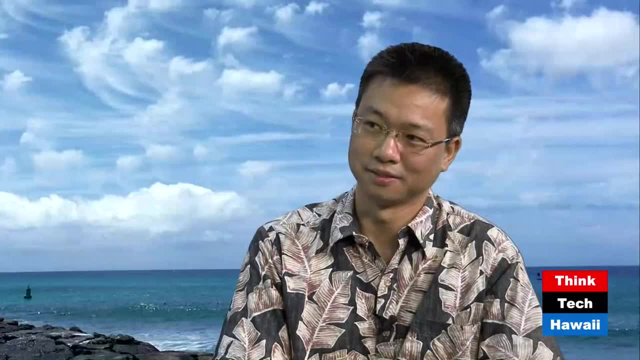 can come out, yeah, and use, but, um, not many, and there were a few other facilities elsewhere outside the United States. yeah, yeah, so there are a few in. yeah, in Europe you have a few in control, but not many, because it's very costly and then need a lot of time. yeah, so that's. that's what I'm talking about. 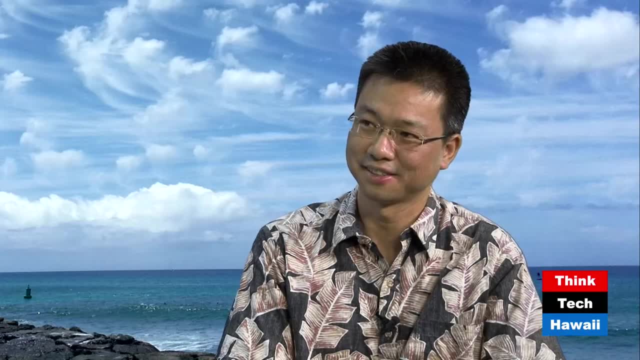 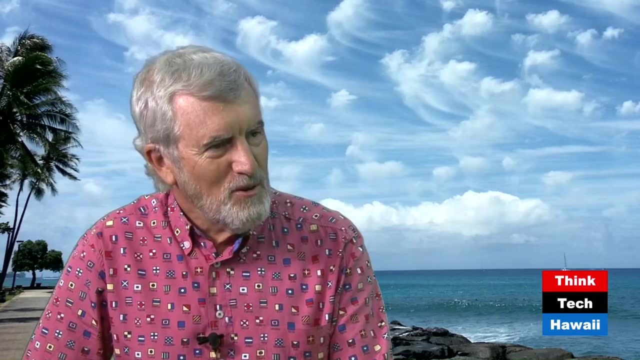 yeah, so that's what I'm talking about. I see. Well, we're just about coming up to a break Bin, but when we come back, first of all I have to ask: why do you do this? It's fascinating. And then also, how did you? 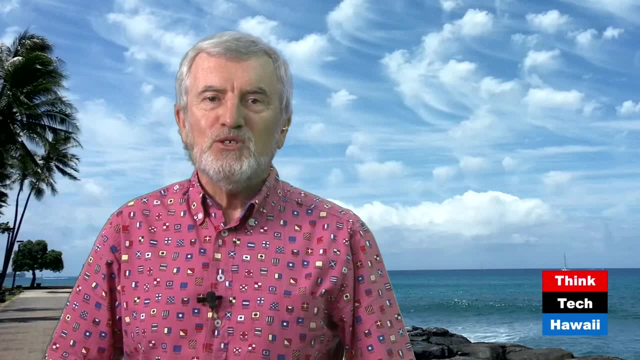 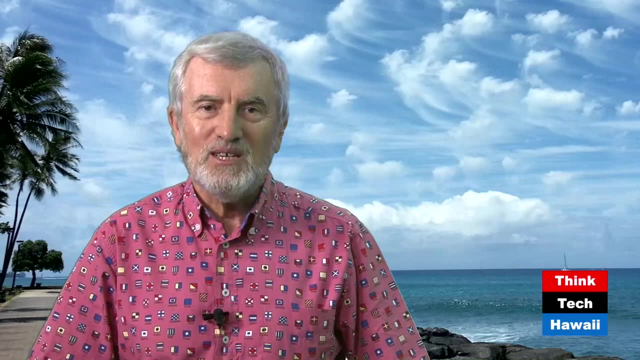 get into this field, So we'll take a break right now. Let me just remind the viewers that you're watching Think Tech Hawaii Research in Manoa. I'm your host, Pete McGinnis-Mark, and my guest today is Dr Bin Chen from the Hawaii Institute of Geophysics and Planetology. 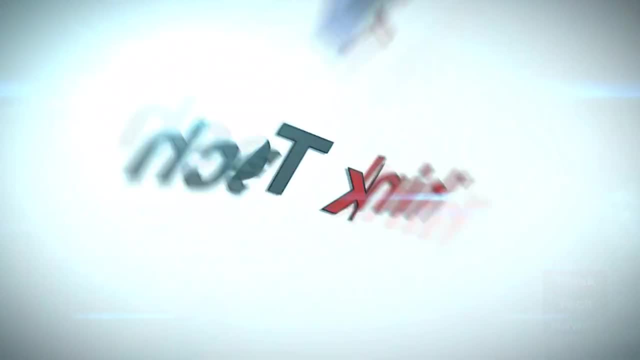 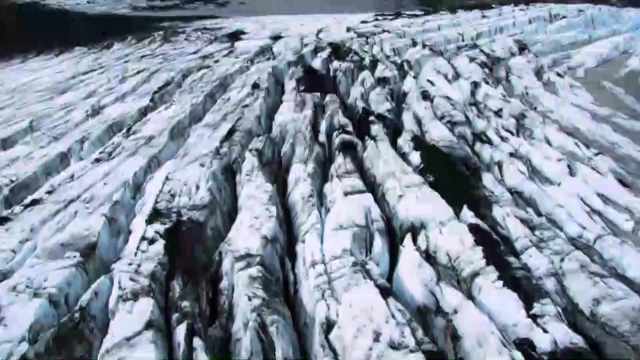 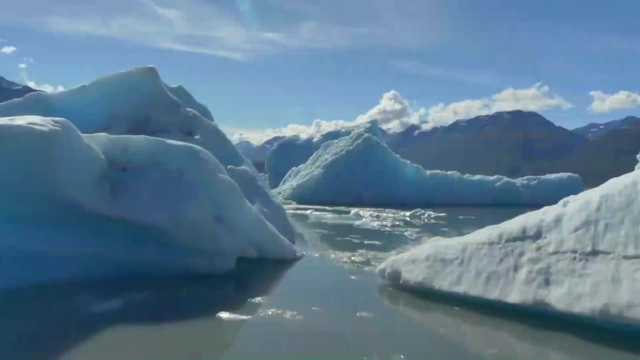 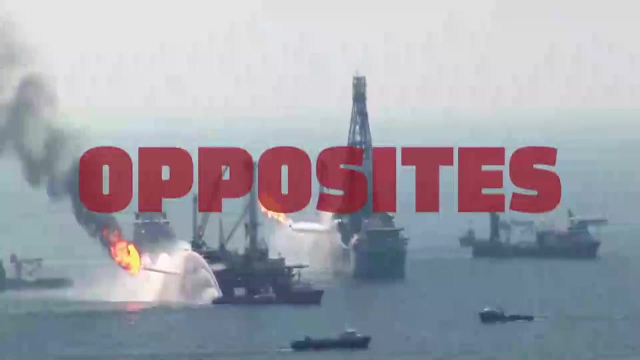 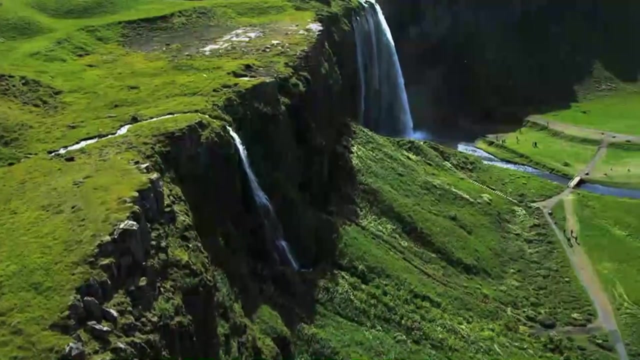 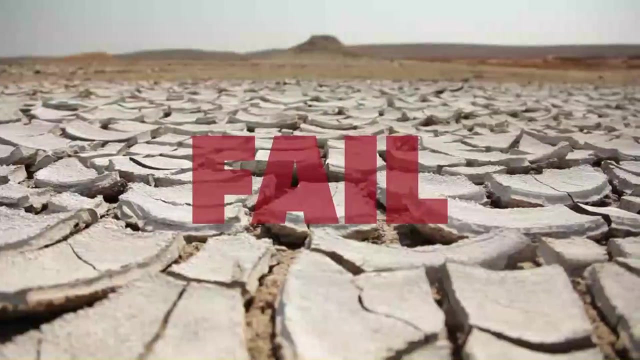 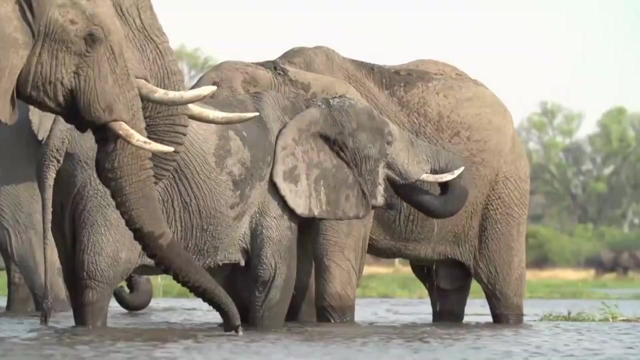 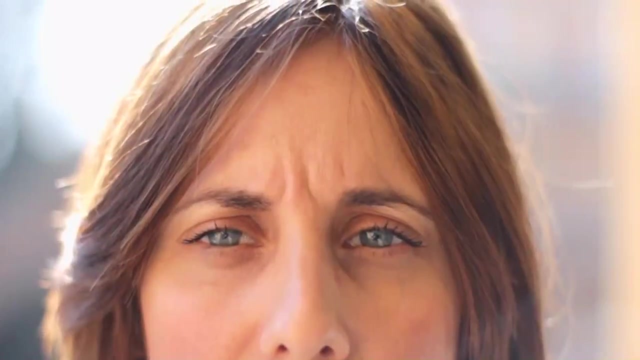 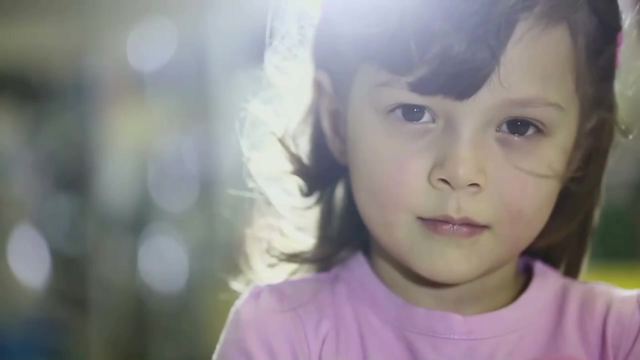 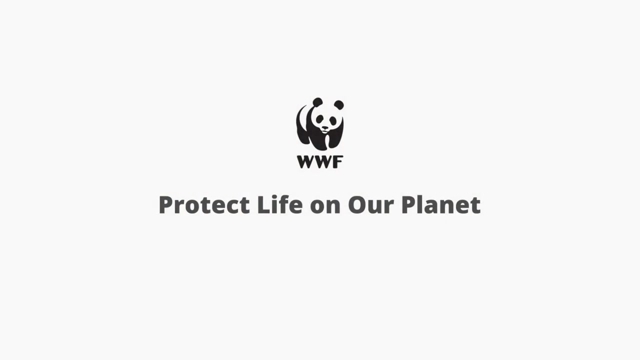 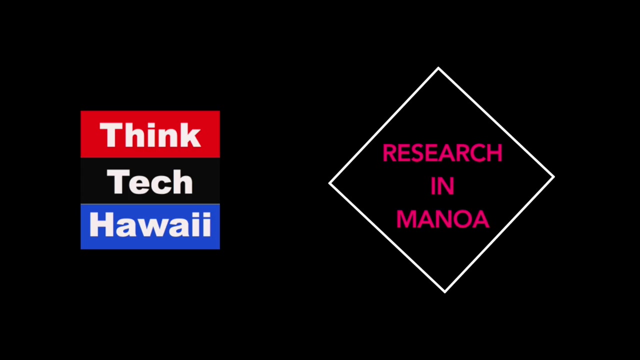 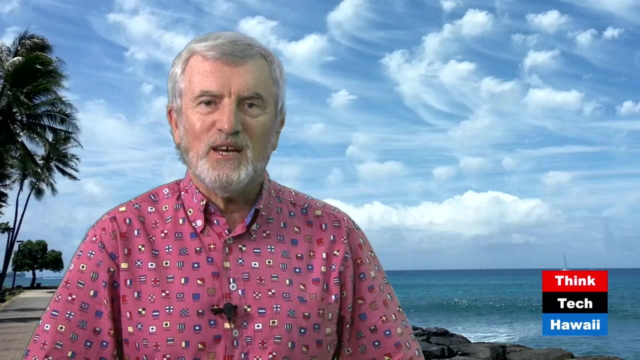 at UH Manoa and we'll be right back. This is Think Tech Hawaii: raising public awareness. Think Tech Hawaii. And welcome back to Think Tech Hawaii Research in Manoa. I'm your host, Pete McGinnis-Mark. 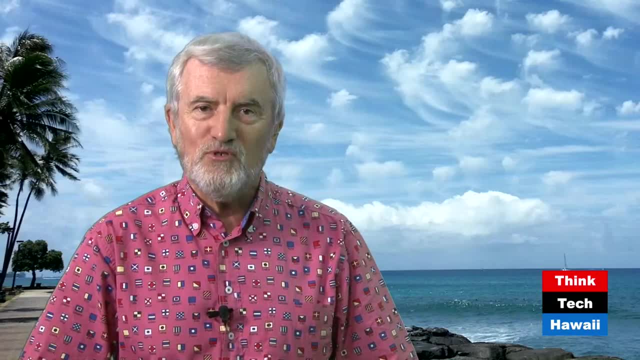 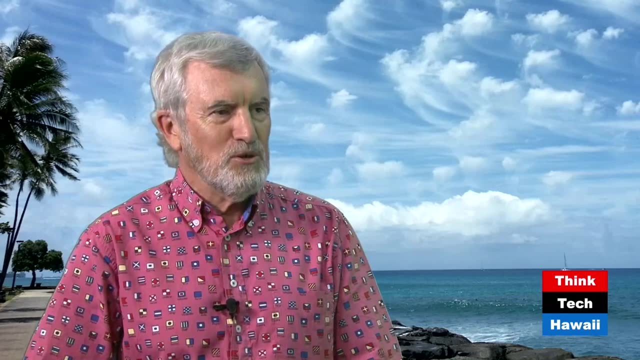 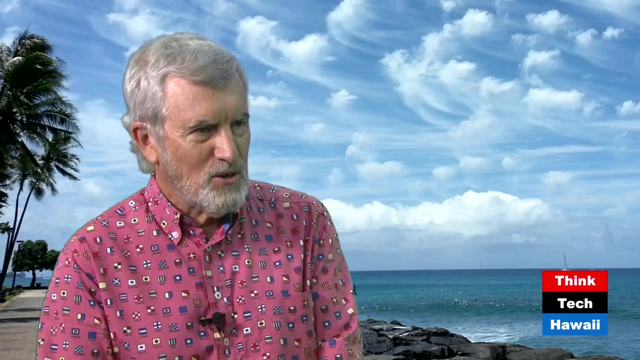 and my guest today is Dr Bin Chen from the Hawaii Institute of Geophysics and Planetology at UH Manoa, and we're talking about high-pressure mineral physics. Well, Bin, before we went to the break, you were showing us slides of some of these pieces of equipment, and I see 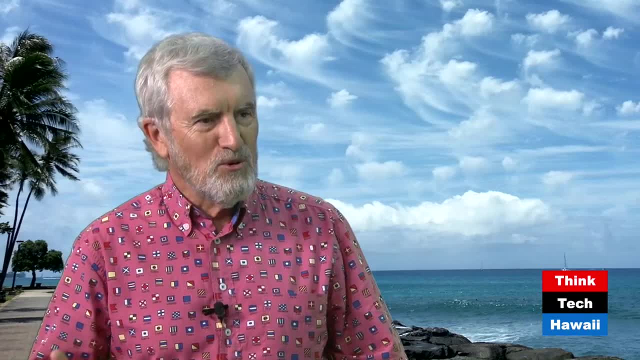 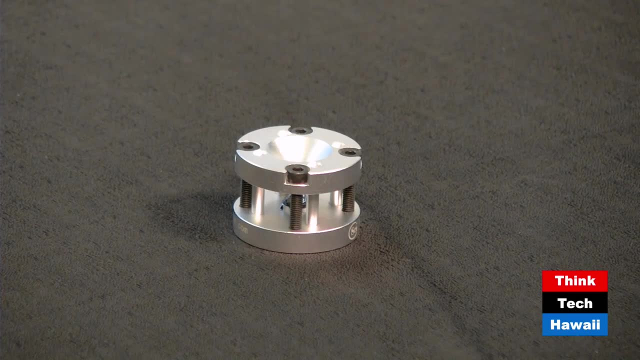 that you've brought to the studio, just one of these small sample holders. So, if we can put the table camera on, what is it that we're looking at? What is it that we're looking at? And let me just put my glasses so that people can see the scale, all right? So this? 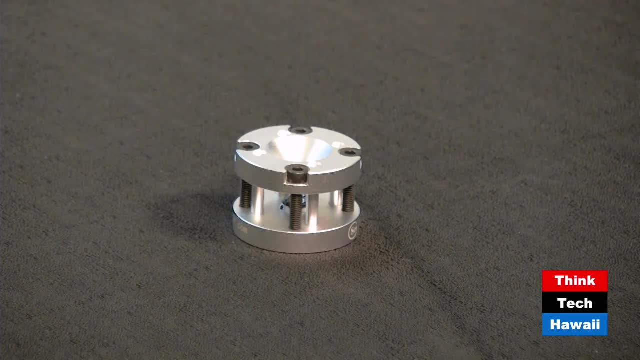 is quite a small little piece of equipment. What is it? So this is a model for the diamond anode cell. So it's pocket-sized, so it can squeeze samples between two diamonds, so between the two curates of the diamond, And then, so we know that. 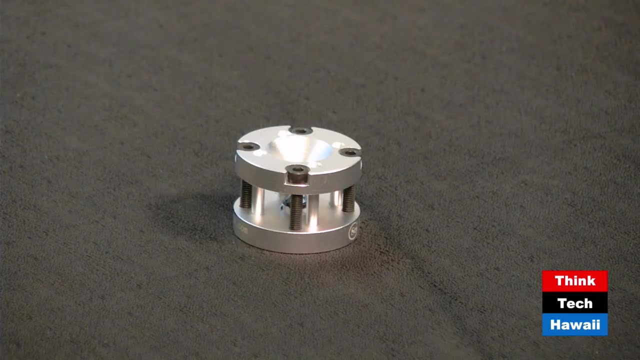 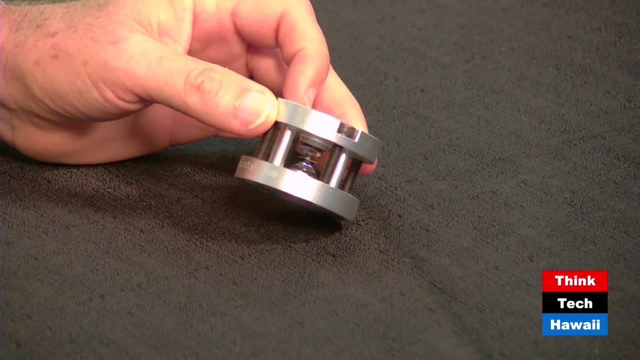 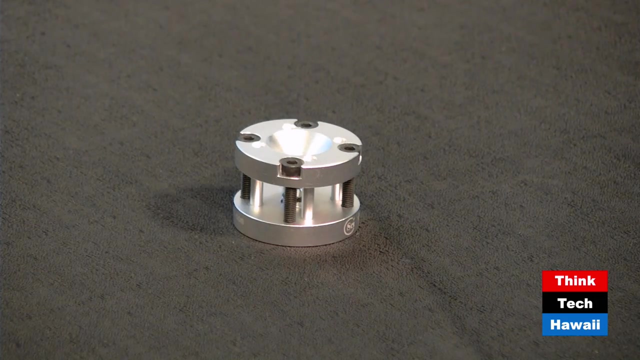 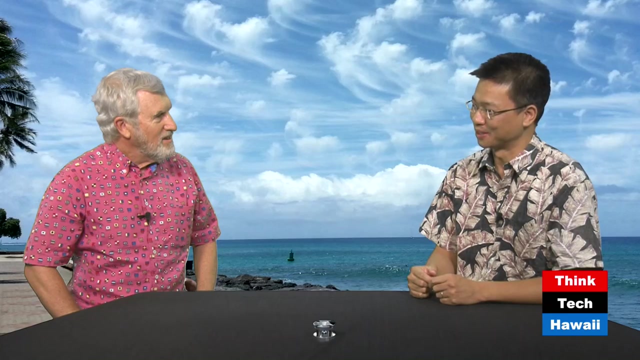 the pressure is generated by applying force to an area. So we've got two little pieces in the middle right. So at the center it's called the metal gasket. So we do a hole in the metal gasket and then we load a very tiny sample in this metal gasket. So of course you need to be quite handy in loading very fine samples to like a curate or like a, you know, like a flat surface with a radius of like 20 microns, Right? So, even though you've got this giant press, that big piece of blue equipment, we 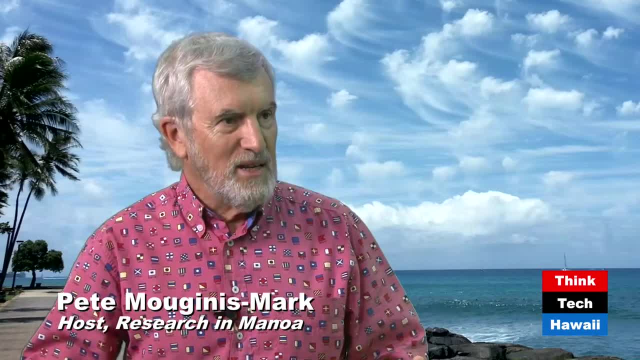 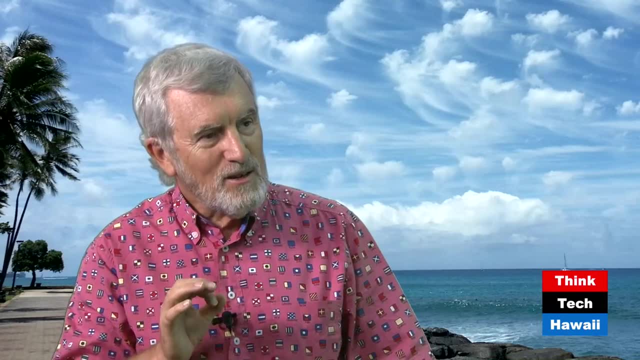 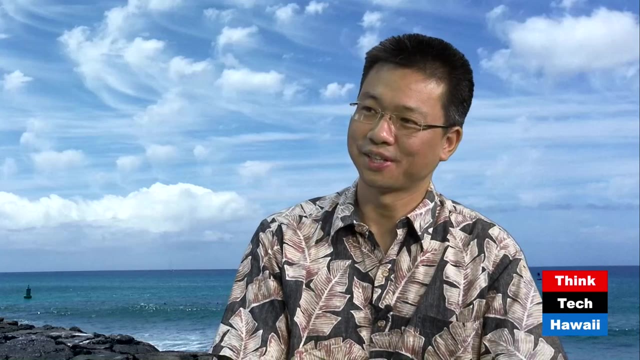 saw in one of the slides, which was, you know, many refrigerators in size. you're working with very fine pieces of equipment. Yeah, So that leads me to the question: how did you get into this field? Yeah, that's a good question. So I was trained as a geochemist. 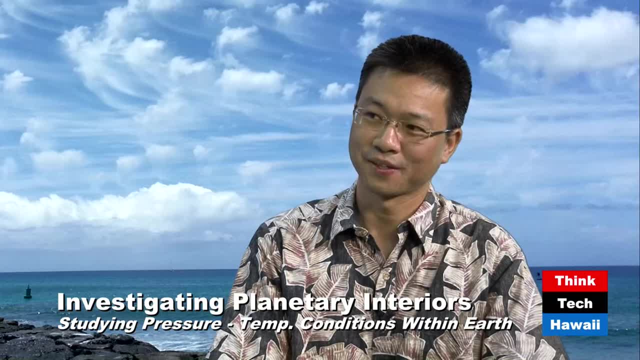 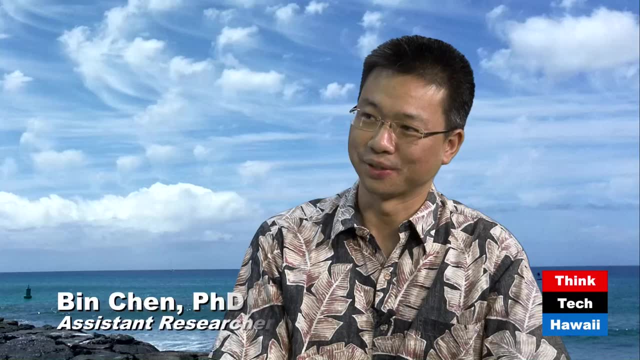 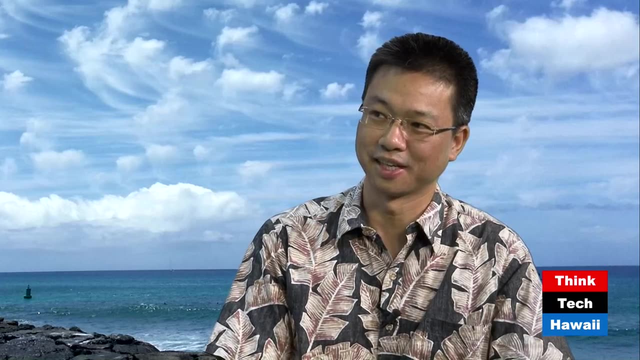 Okay Before. So I worked on oxygen isotopes of metamorphic rocks, Okay, And when I applied for graduate school, so I yeah happened to enter this field and I like it because I like to get my hands dirty in the lab. and then yeah, and then I think 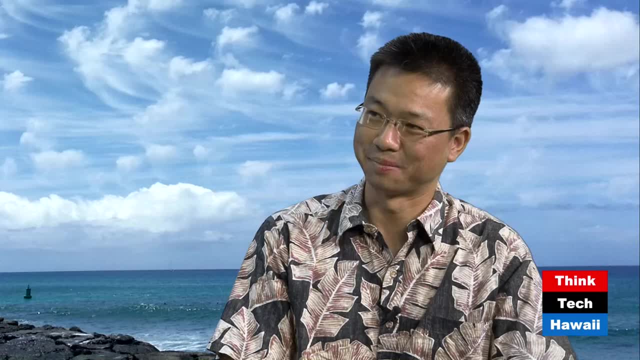 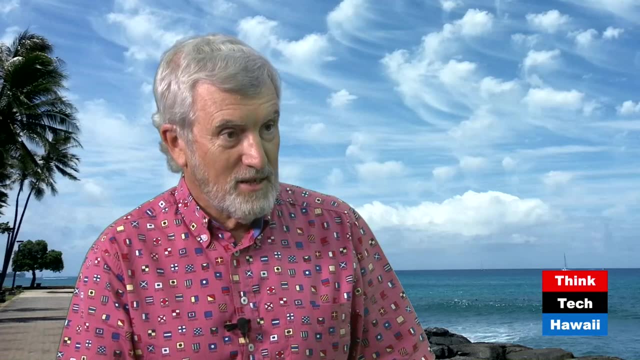 I'm quite good at like doing all these experiments, So I'm always fascinated with people's career paths. Yeah, And I think, as a geologist correct. Yeah, geochemist, yeah, Geochemist, you were looking at the composition of different rocks and 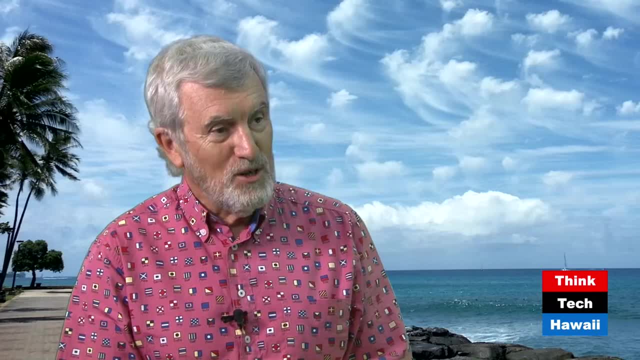 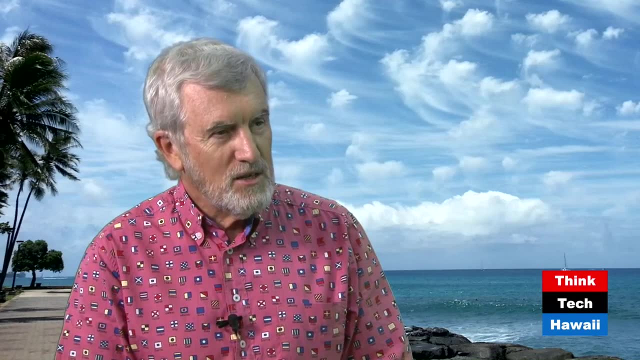 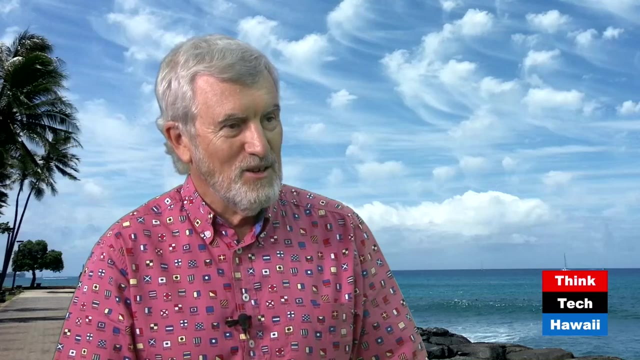 And the isotopes- The isotopes of this material, But then you seemed to be into equipment and doing really fine detailed stuff. Did that transition occur when you were in graduate school or when you applied to UH for a job? Have you been doing this for years or? 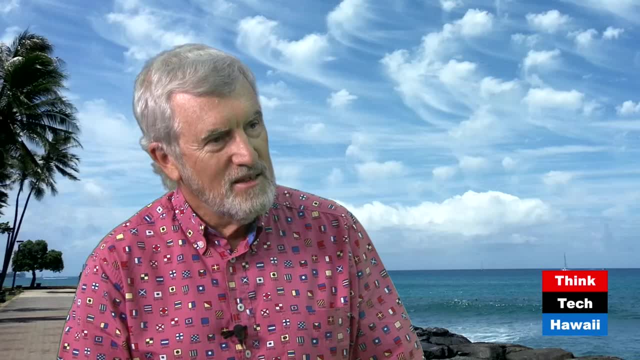 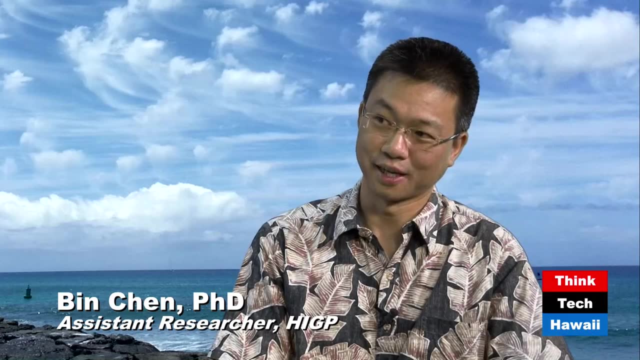 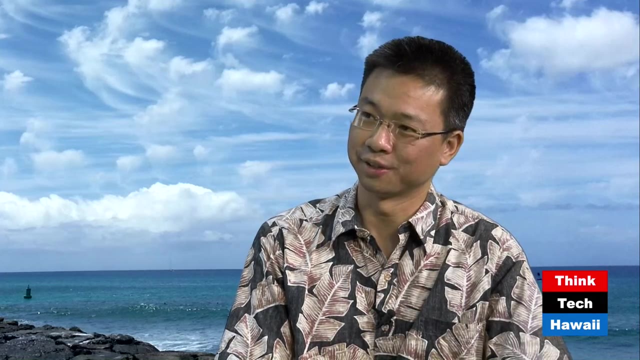 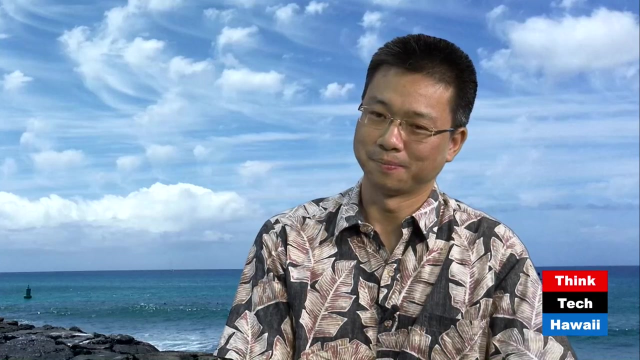 Yeah, I have been doing this for years. I have been doing this since 2004.. Actually, my first project is about Mercury, The planet Mercury. Yeah, the planet Mercury. So we conducted a high-pressure experiment on the melting of the iron-sulfur system and then we found that, like the snowing or raining of the 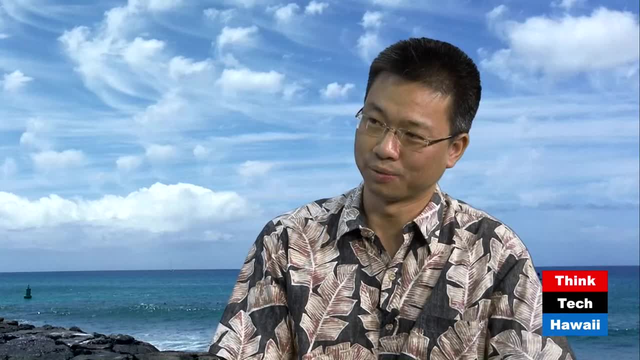 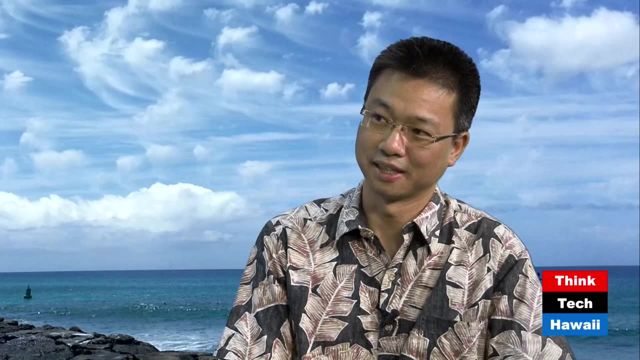 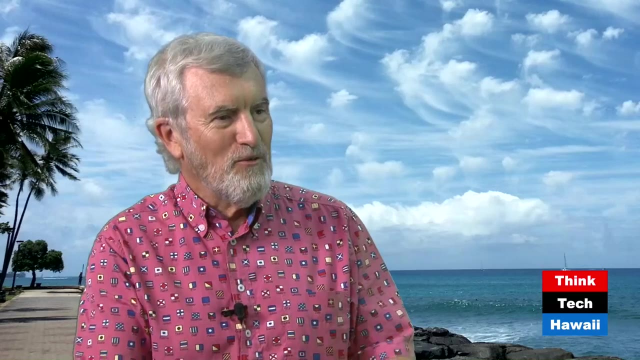 iron crystals in Mercury's liquid outer core. Okay, Yeah, And that's how we found out that the magnetic field in Mercury is possible- is likely the cause for the magnetic field in Mercury. Would you say your career path is unusual. If someone wanted to follow you, would she? 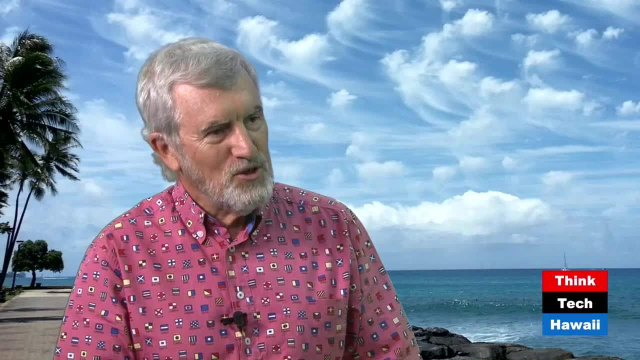 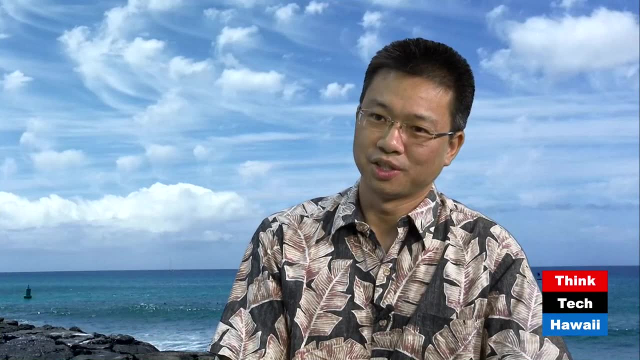 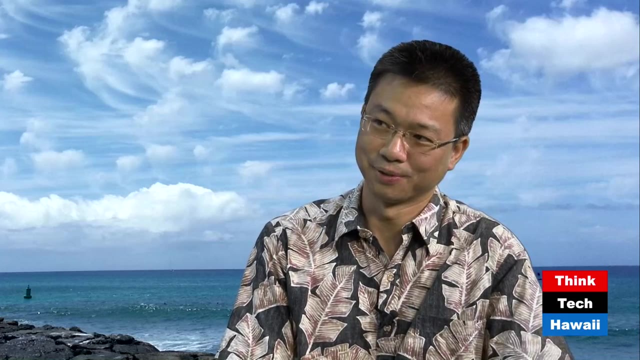 be able to do this kind of study at any university, or is there just one or two places around the country which specialize in Mineral physics program is not a very large program in the US. Yeah, Only like a handful of- yeah, a handful of like universities have this program. 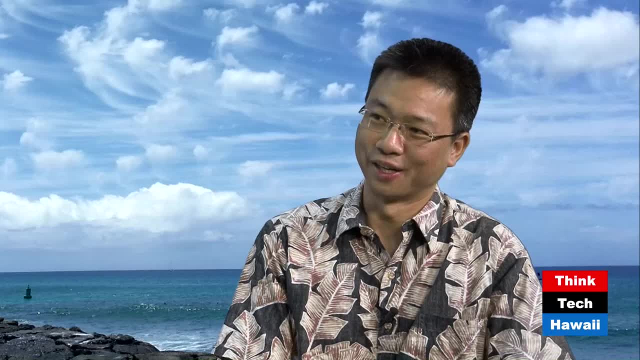 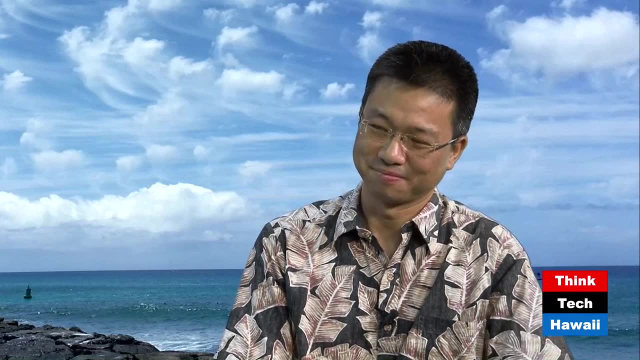 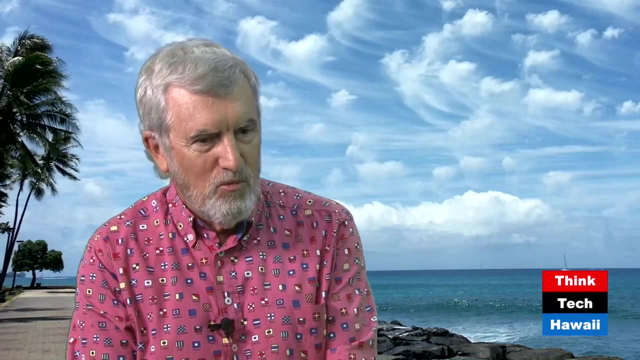 And I think it's not a like unusual, like career path. Yeah, It's quite unusual, Yeah, But then the next question is: why should anybody care, Mm-hmm, What would the person in the street see as the relevant? 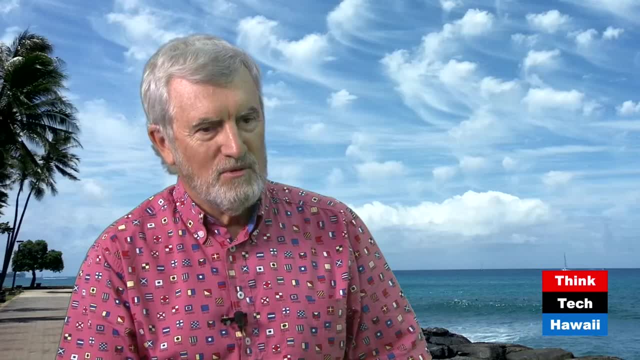 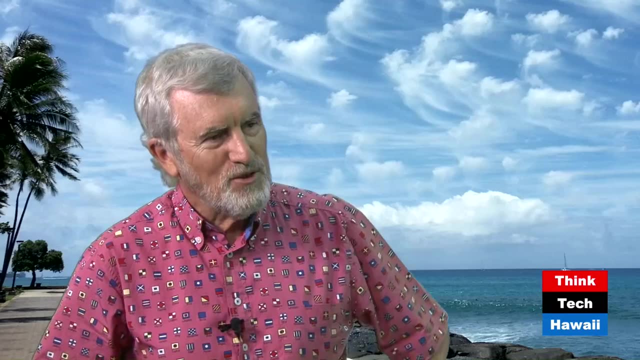 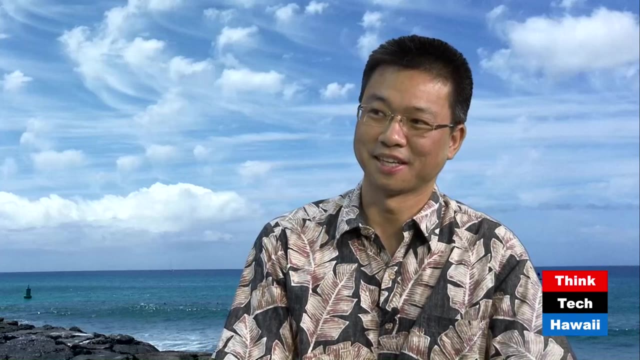 What's the relevance of this work? How do you justify studying these minerals at extreme pressure? What's the relevance? Yeah, The main reason is out of curiosity, Like all these space machines. So we send the spacecraft to the outer space and then trying to understand the universe. 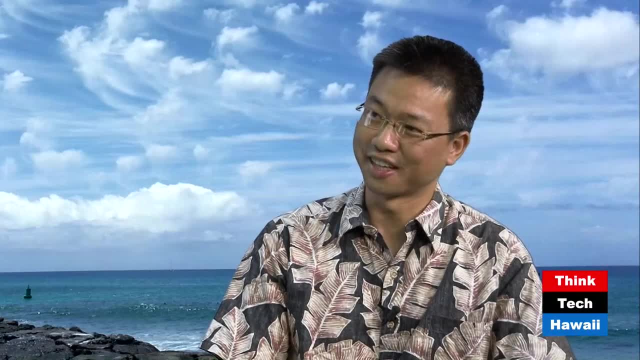 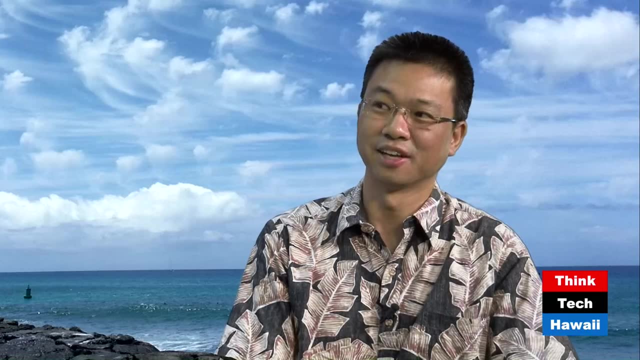 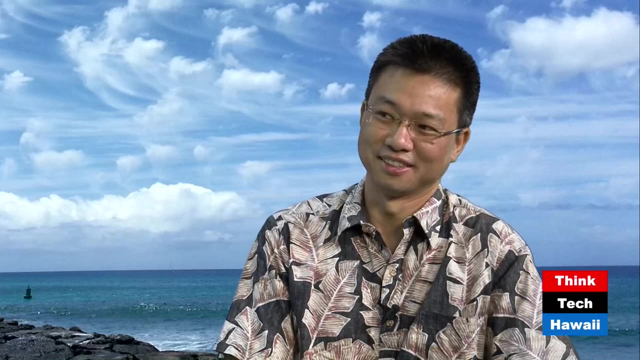 right. Actually there is also a universe in the interior of the planet, because it's actually more inaccessible than the outer space, Because you cannot drill a very deep hole through the interior of the Earth, I think, and then you get the sample. 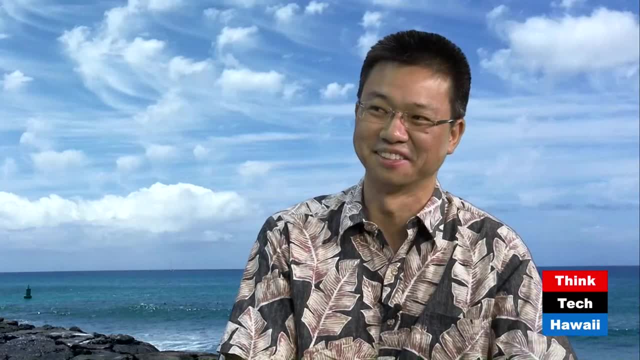 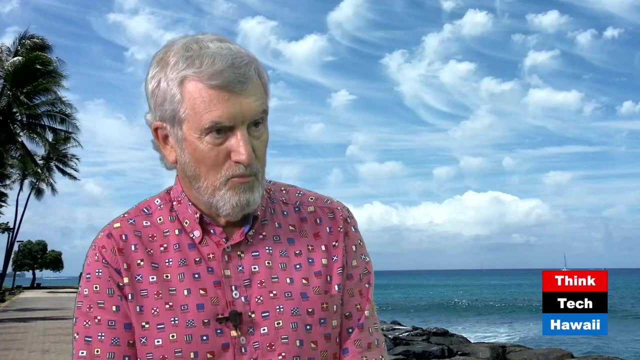 But it's probably easier to get a sample from the moon than you get a sample from the. So the work you do is kind of a detective story, trying to understand where particular minerals occur within Mm-hmm, Let's say the Earth's interior. 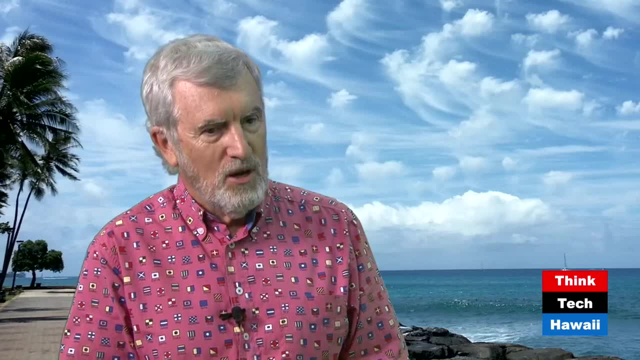 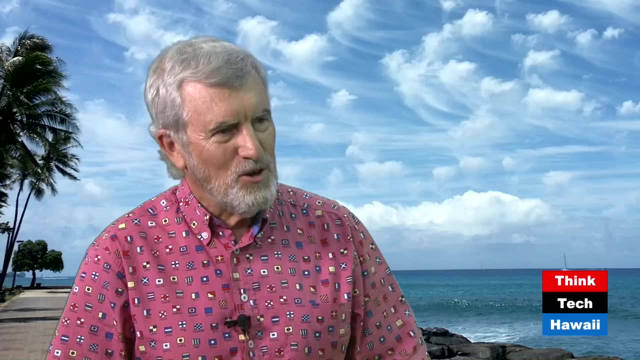 Mm-hmm. Is that important, You know? is there anything Mm-hmm- I've heard that you know- sort of earthquakes. the shock wave can go Mm-hmm through the entire interior of the Earth. 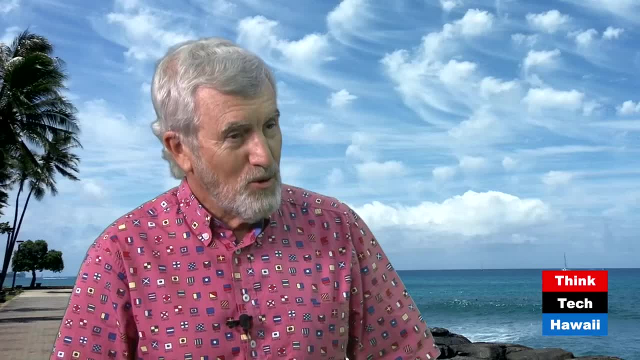 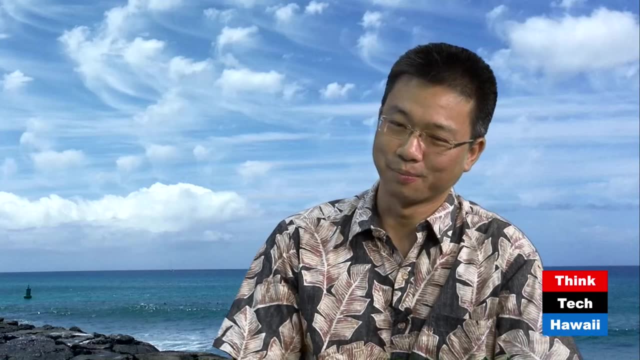 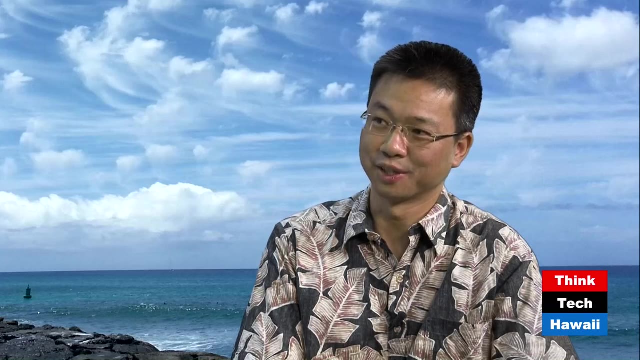 Mm-hmm, Does your work relate to understanding earthquakes or My work is not directly related to earthquakes, but my colleague, so our colleague, So he's now Mm-hmm, He's now working on the subducted slab, like some of this mineral. 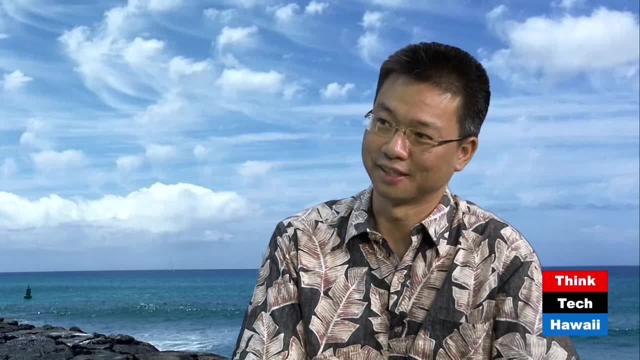 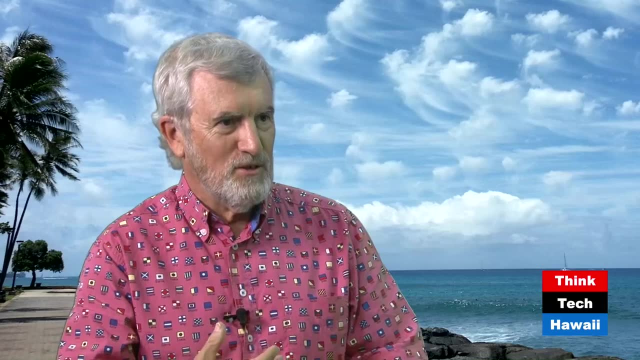 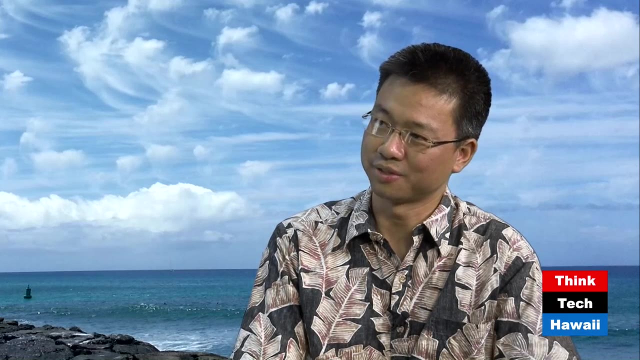 Some of the minerals found in the subducted slab. Okay, And like Subducted slabs is where the Earth's crust is overturning through plate tectonics. Yeah, Yeah, yeah, And my work is So. we are trying to understand the physics and chemistry of the planetary interior. 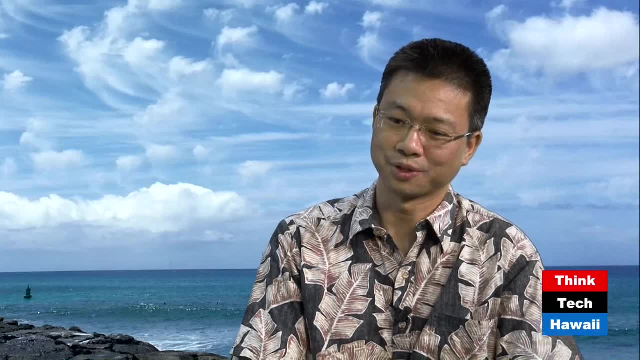 Mm-hmm, And So, of course, the main reason. So of course the main reason is about: Yeah, it's out of curiosity, Like curiosity. And then the other is actually we. Our research is a very important piece that we can use to understand the chemical evolution. 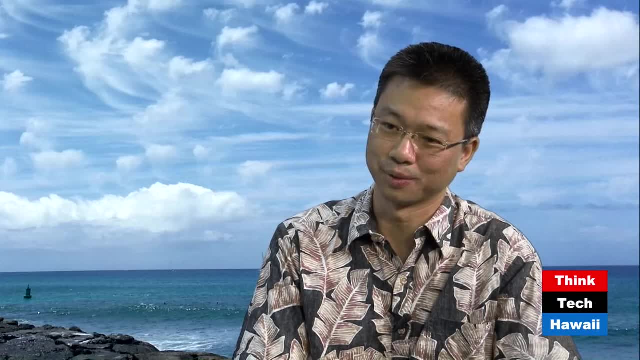 of planets, Like if we look back in the history of the Yeah over planets and how all these- And I've also heard that you know the Earth's interior is probably Mm-hmm. Yeah, Yeah, Yeah. 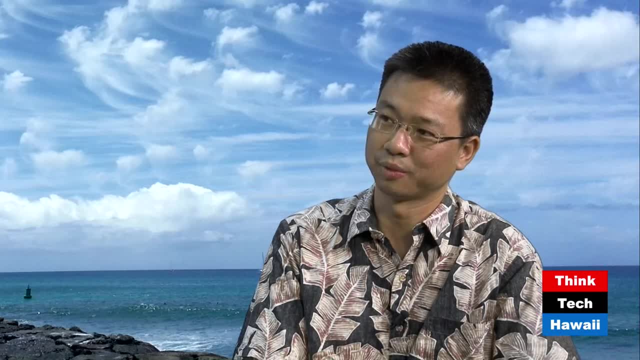 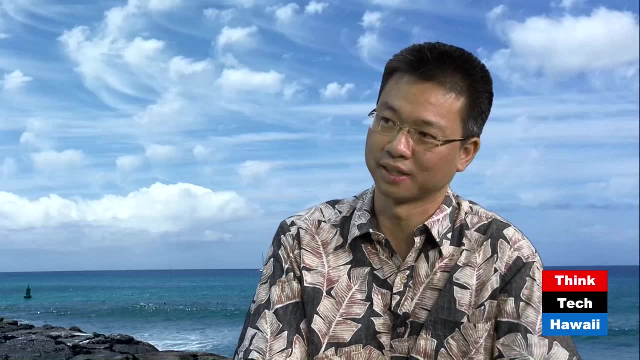 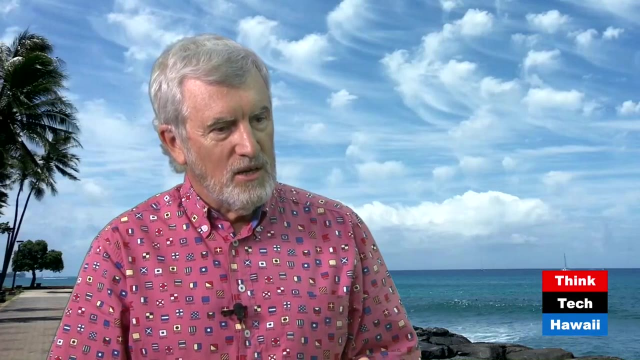 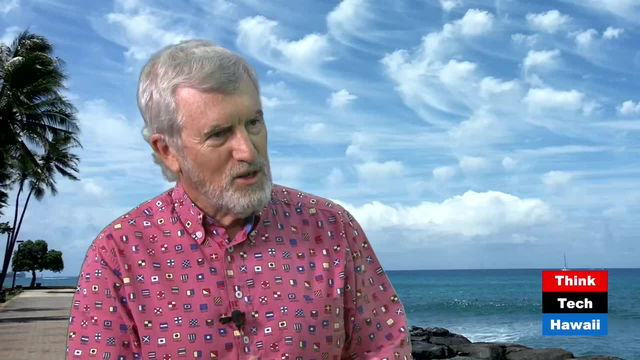 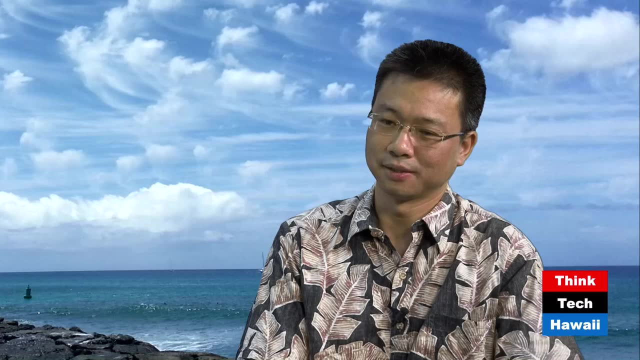 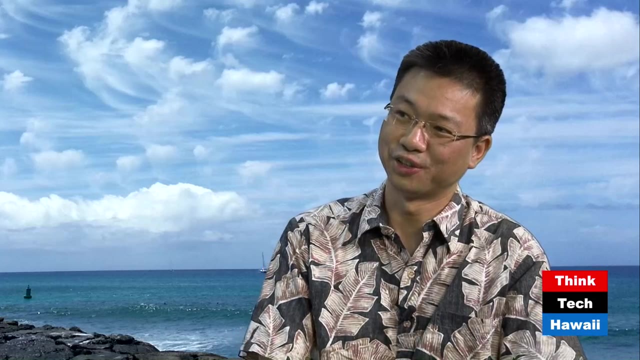 us from radiation Mm-hmm. Is that correct? Does that relate to the kind of work that you can do? Yes, So that's So the work I did for About the Mercury score. So Mercury is a very smaller version of Earth, right? 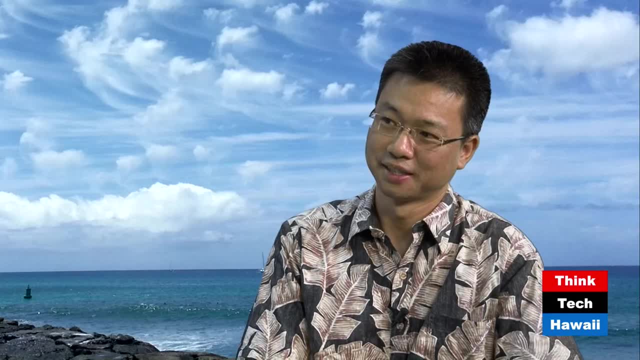 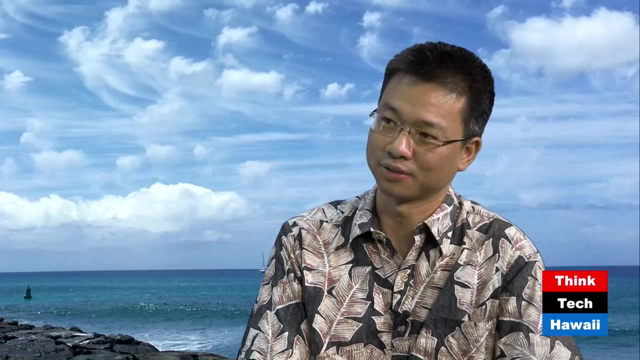 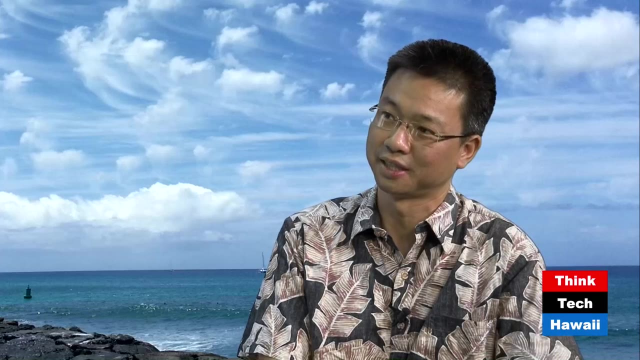 Yes, So Mercury also has a magnetic field. So our work, Oh well, Our high-pressure work- we propose a very good mechanism for the generation of the magnetic field in Mercury, And I hope that we can do the same for the Earth. 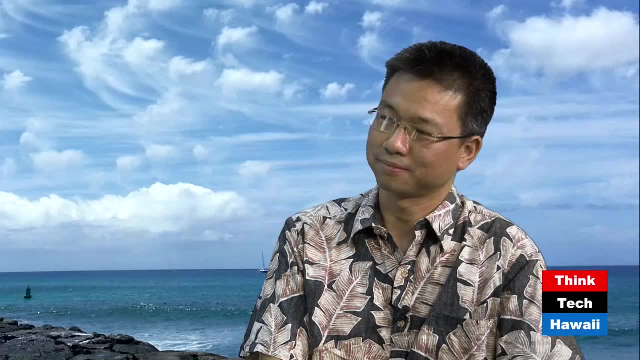 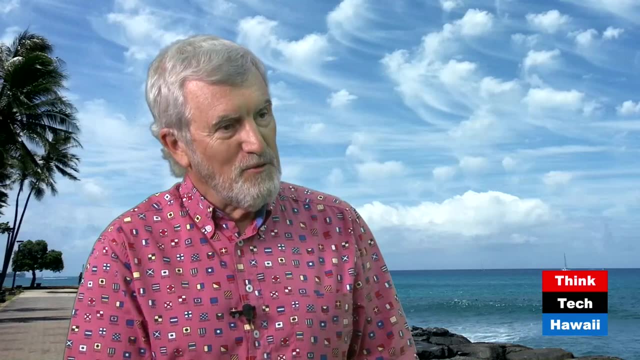 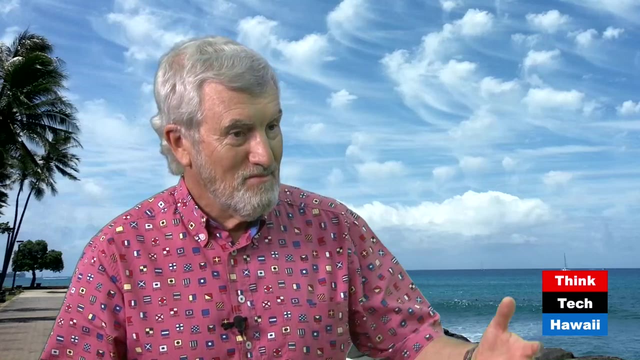 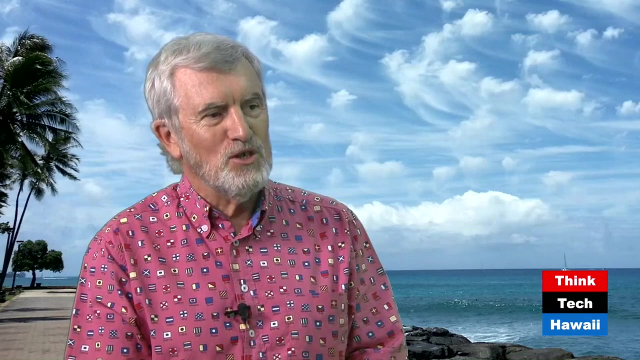 And even planets like Jupiter have magnetic fields which Jupiter's interior is at much higher pressures, And the magnetic field is of relevance to people in their everyday life because it shields us from The radiation from the outer space. I see So that, even though your research is basically pure discovery, 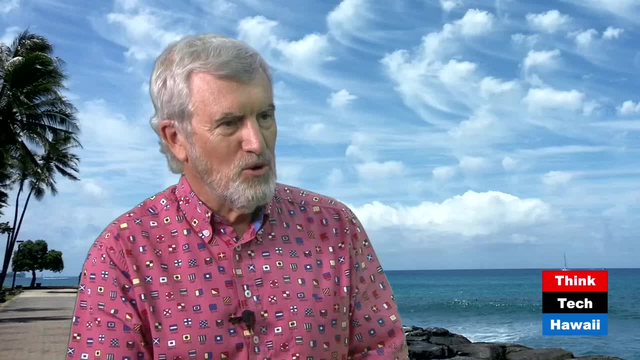 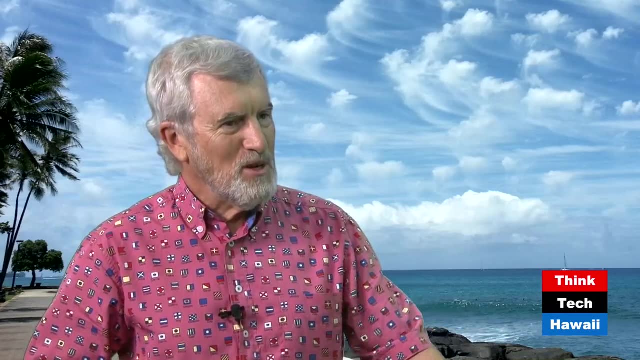 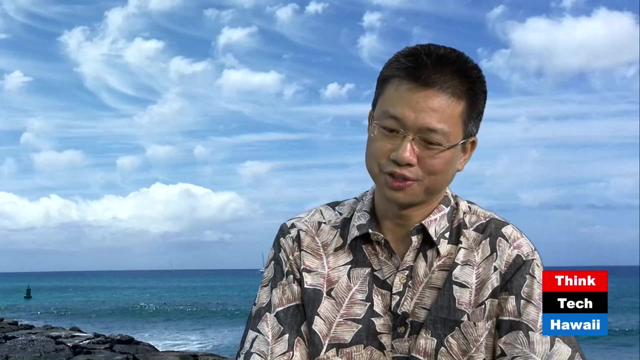 there are things like studying deep earthquakes, like studying the magnetic field which protects us from the Sun, So that's presumably why NSF is interested. is that correct? Yeah, And also our research. there might be some byproducts from our research. 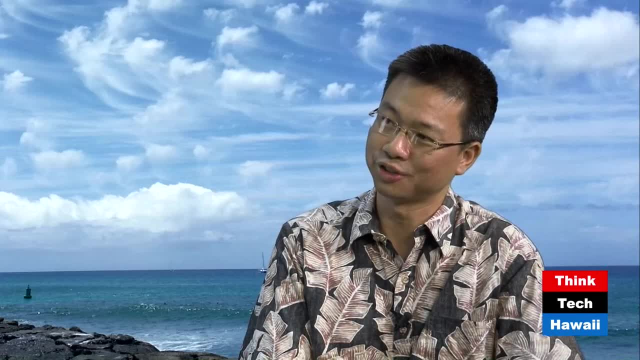 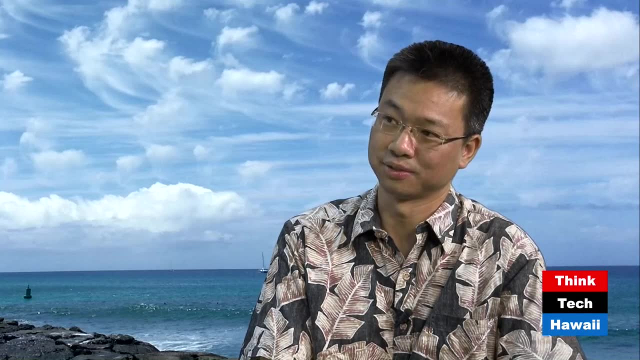 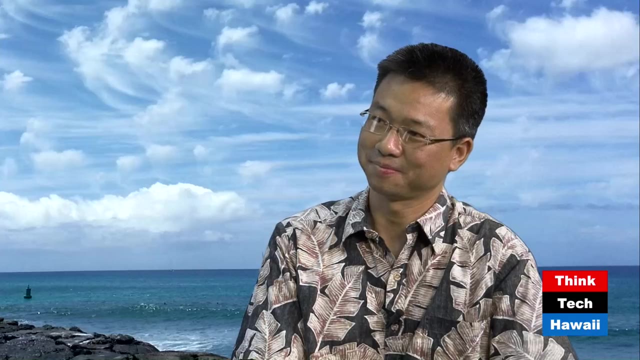 For example, some group of researchers. they think that there's a large nanocrystalline diamond that has industrial use. Ah, so you mentioned diamonds, And diamonds are created deep within the Earth, Deep within the Earth's interior, So you can. 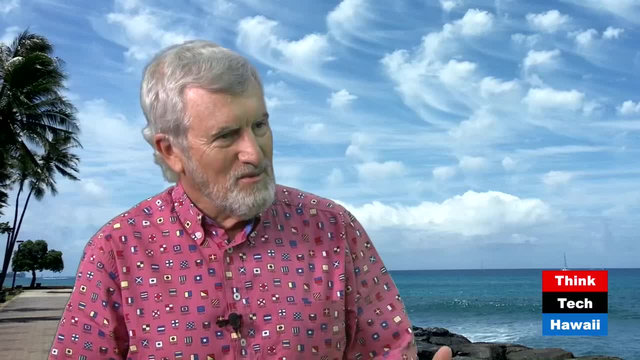 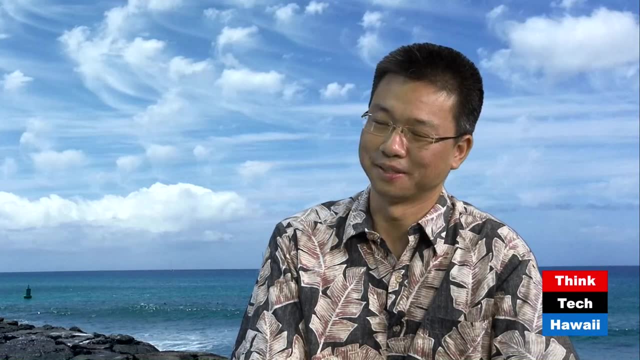 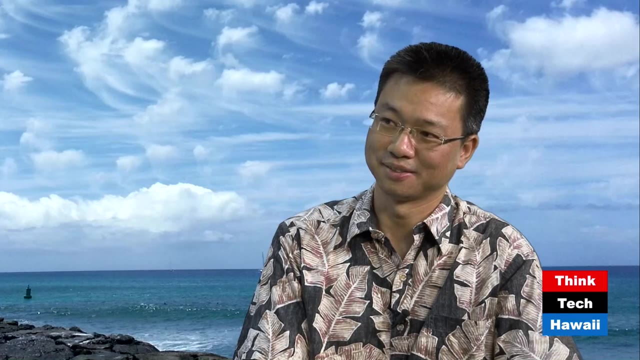 Can you make diamonds? Can you sort of The pressures that you're producing? Yeah, we make diamonds all the time Because if we use a graphite capsule and then under pressure and temperature, like produced by our multi-ample press, so we can sense those diamonds very easily. 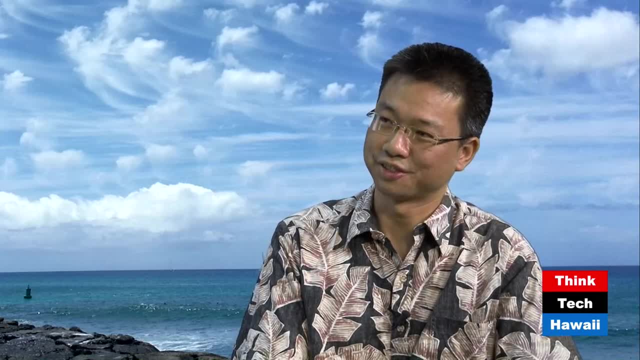 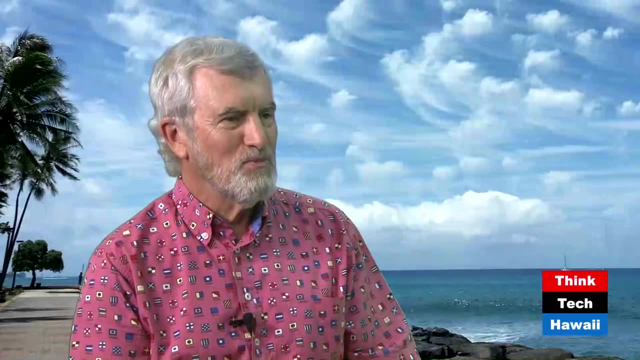 Yeah, Okay, But of course, if we want to synthesize like a centimeter-sized diamond, then we need a larger press. Okay, So you're not going to get rich by mass-producing diamonds then I mean, some companies are doing that. 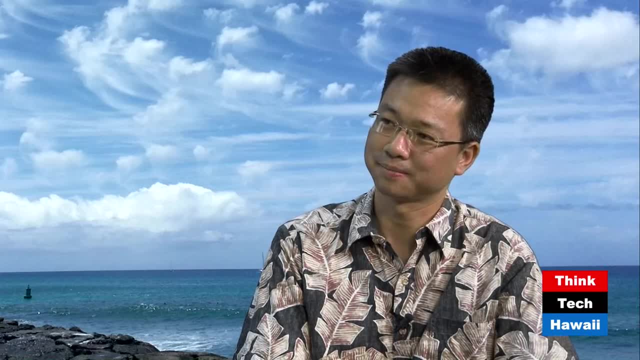 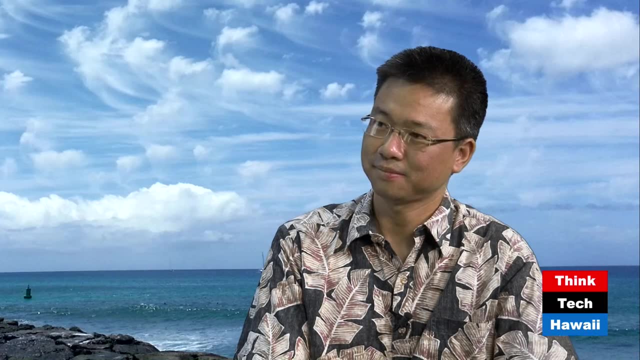 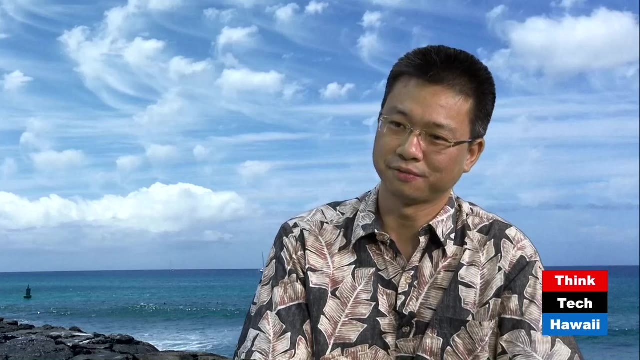 Are they really? Yeah, they are synthesizing some like diamond. So are there commercial applications trying to understand materials or anything like that? Yeah, I think. So, these high-pressure techniques. so we use it for basic research, but we can also use it for material science research. 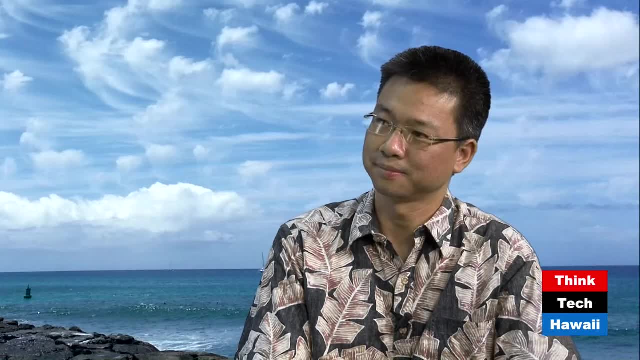 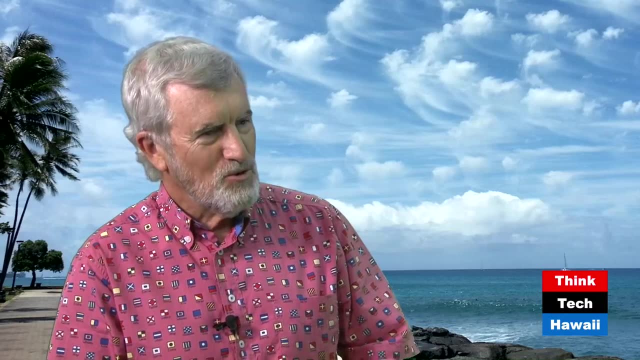 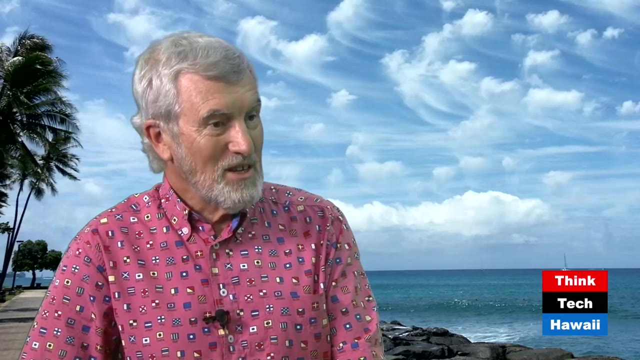 I see And I've heard of other faculty members at UH who have actually looked at the performance of material under stress, either in explosions or that sort of thing. So there's a lot of relevance, even though you're basically doing pure research. 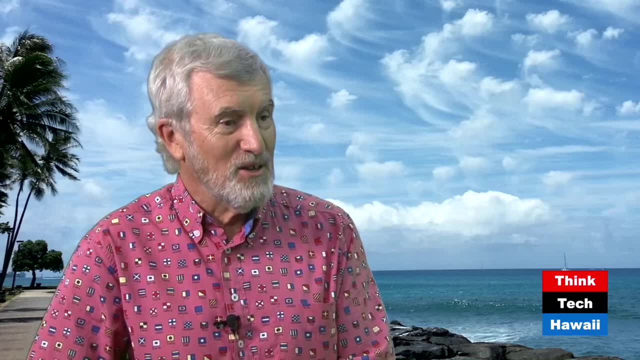 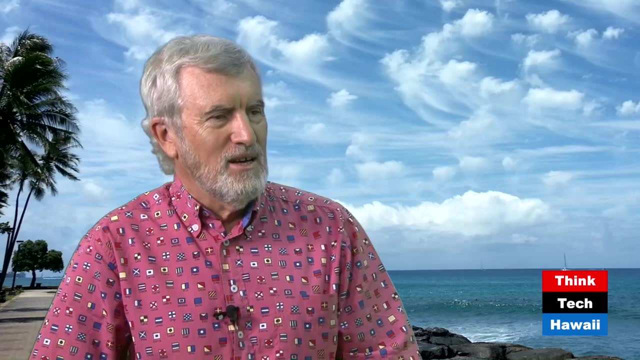 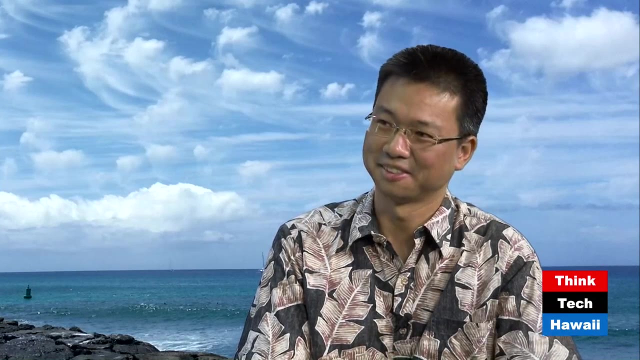 as we've found in this show and many other programs, The pure research has direct relevance either to people in Hawaii or to the broader society in terms of new technologies and that sort of thing. Yeah, That's terrific. Well, we're getting near the end of the show, Bin. 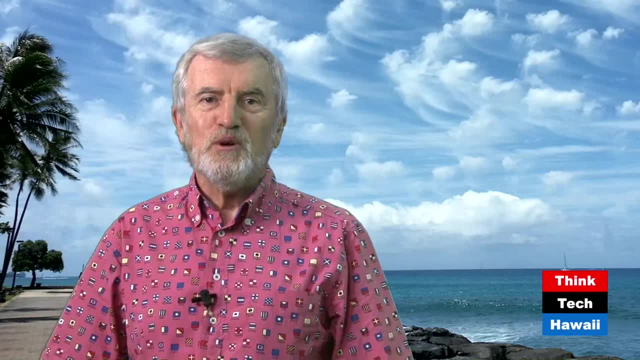 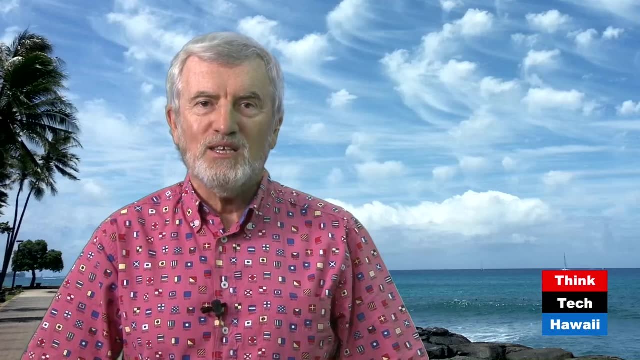 So let me just thank you again and remind our viewers: you've been watching Think Tech Hawaii Research in Manoa. I'm your host, Pete McGinnis-Marck, And today we've had as our guest Dr Bin Chen, who's an assistant researcher at the Hawaii Institute of Technology. 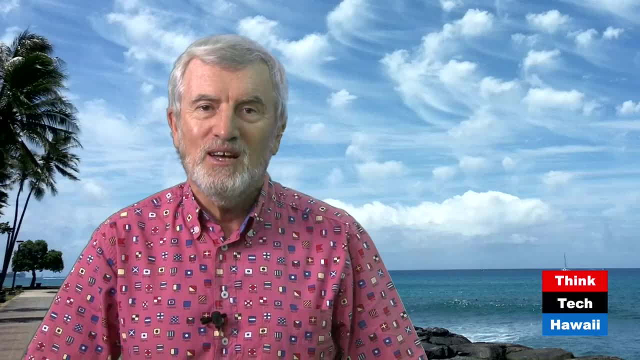 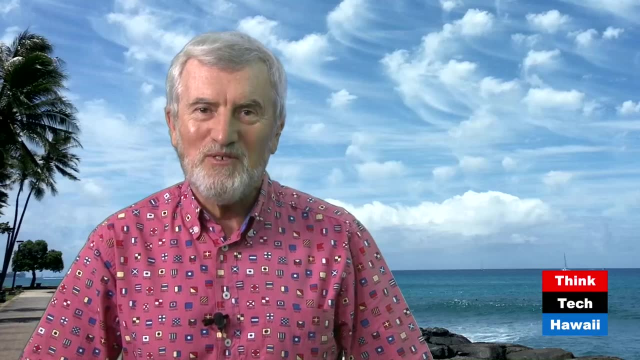 Dr Bin Chen is an associate researcher at the Hawaii Institute of Geophysics and Planetology at UH Manoa, And thank you for watching today And hopefully you will join us again next week at the same time. Goodbye for now. Thank you.